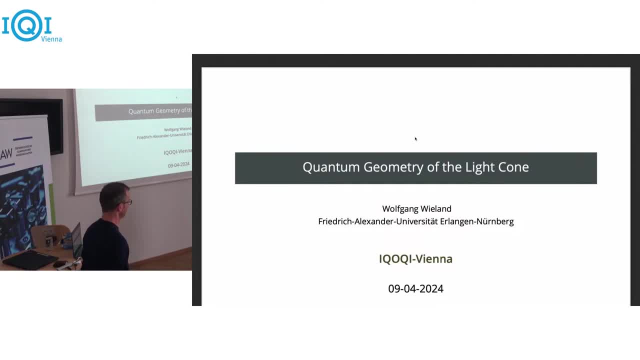 For his work in quantum and gravity and spin forms in 2019.. And also a special prize for his PhD. And he was known for his work in quantum gravity- general quantum gravity and classical gravity and quantum conditions. And today we heard something about quantum geometry of the light. 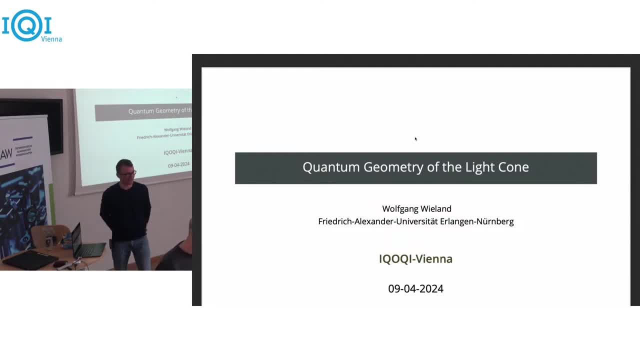 Thank you, Csárdá, for the very kind introduction, And it is really nice Being back here in Vienna. And yeah, today I would like to speak about something that I have been thinking about for a long time, in fact, and wanted to do in different ways and experimenting different truncations, different techniques. 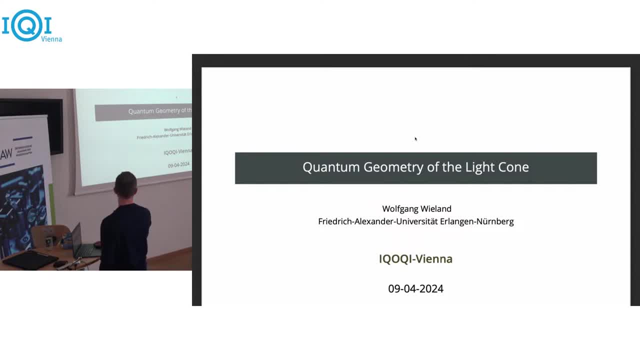 And I think now I have some interesting result. Actually, there may be a problem with my pointer, but that's not an issue. That's not an issue. That's not a problem. I think there's on. maybe I should put on. 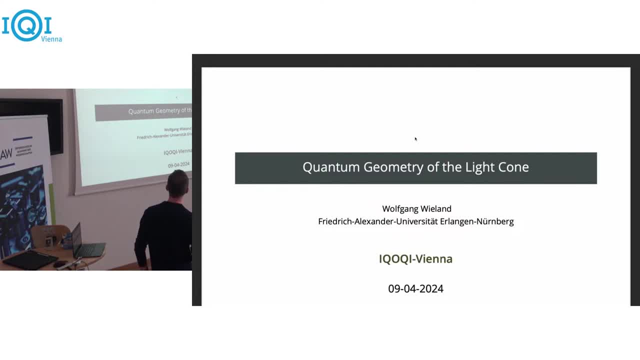 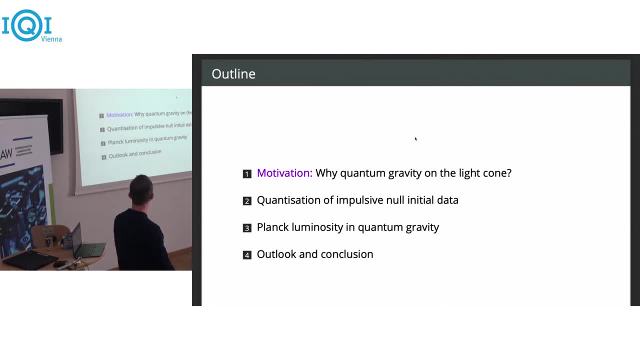 Okay, So now it works. Okay, so the talk is about the quantum geometry of the light form, And let's start out with a basic outline. So first I will give you just a very brief motivation for what I want to speak about. 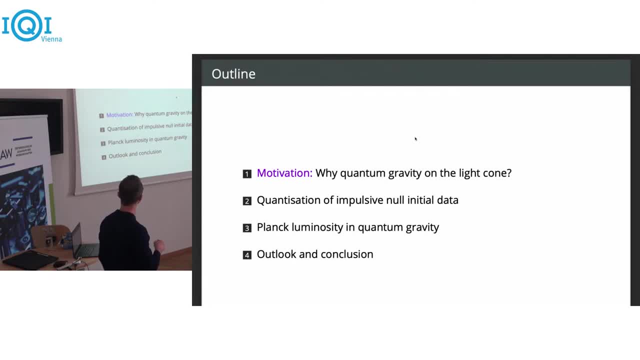 And then I Speak about also the quantum theory, And then there seems to be something interesting happening, namely I can speak about luminosity. So you know, for instance, a gravitational wave signal emits a certain energy per time. This is called in astronomy, luminosity. 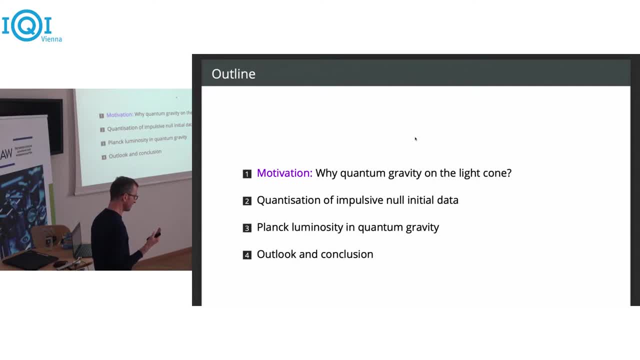 And but in if we, if we take into account that there's H bar G, Newton and C- the speed of light, we can build natural units. So out of the Planck, namely the Planck length, Planck units, and out of Planck mass and Planck time and speed of light, we can get a Planck power, Planck mass times, C squared divided by Planck time. 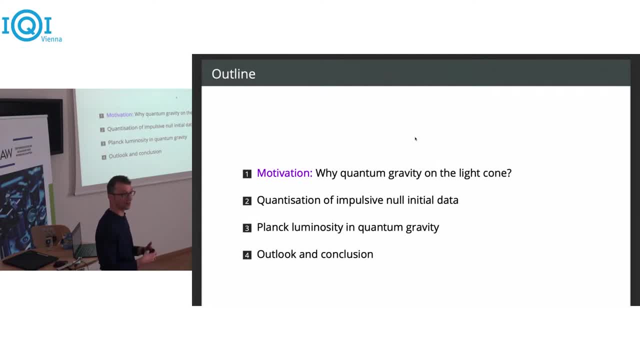 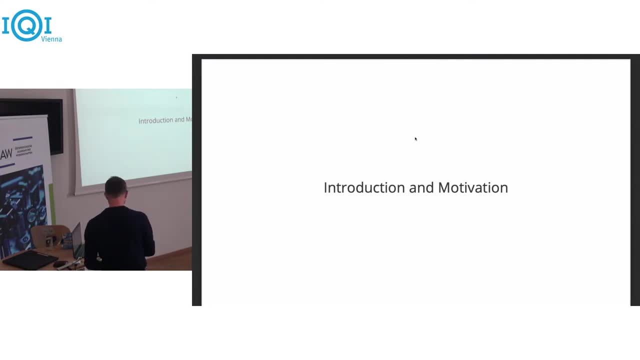 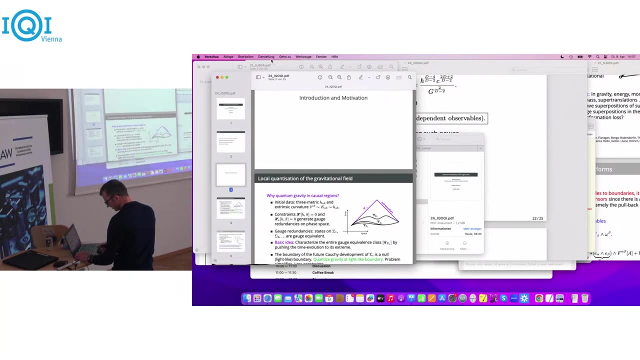 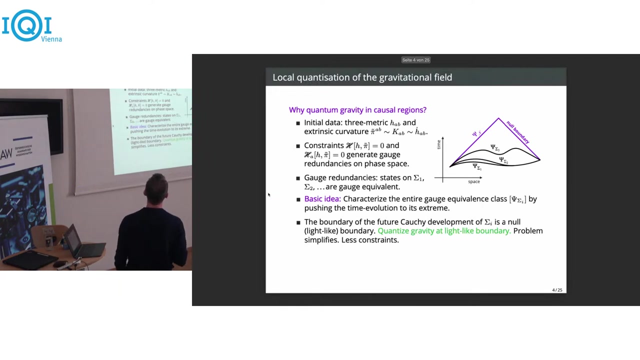 And it seems that in this quantization the Planck power plays a certain role And it's. this seems exciting to me, And it seems exciting to investigate. But let's first go into the basic introduction. That's better. Let me give you a basic motivation for what I'm doing. 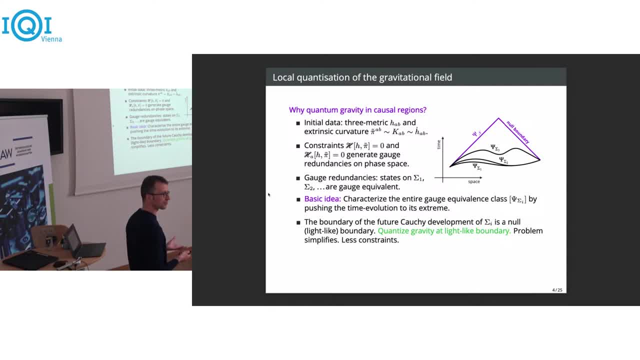 So in a quantum state represents the quantum Analog of a classical state. of course, classical states are points on phase space in general, relativity. phase space is space space of initial data, and initial initial data for gravity is the three metric on a Cauchy surface and the extrinsic curvature, which is basically the time derivative of the metric. 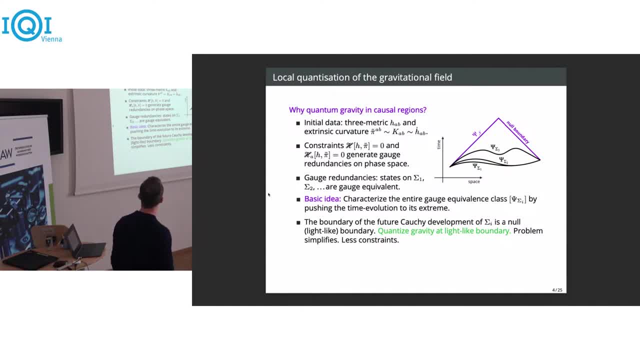 This is like in mechanics: Q and Q dot initial data for your particle, Particle motions. but then general relativity is different from mechanics because it is a gauge theory and the there is. there is a gauge in variance and this is, if you morphism in variance, in fact the constraint. the initial data is not arbitrary. so not any three metric and extrinsic curvature will be compatible with the solution of the Einstein equations. 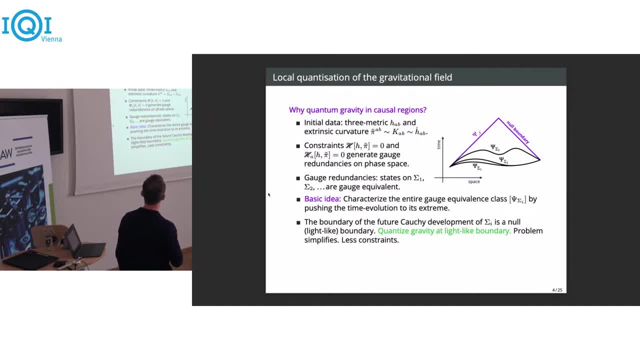 You have to impose constraints, namely a scalar Constraint and the vector constraint, and these are dual to vectors: vector fields in space time that generate that generate the few morphisms. In fact, they generate the few morphisms only on shell, if the constraints are satisfied. 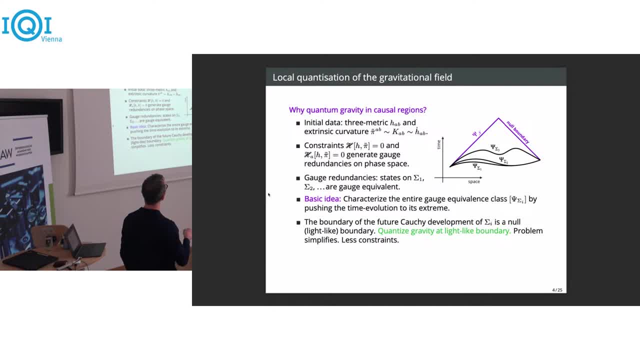 But what that means is that if we start out with some initial data that satisfies the constraints, Then generate the solution to Einstein equation, But then choose a different hyper surface, we get new which is related to the first one by the few morphism. we get new initial data, but these new initial data will will be just gauge equivalent to the original one. 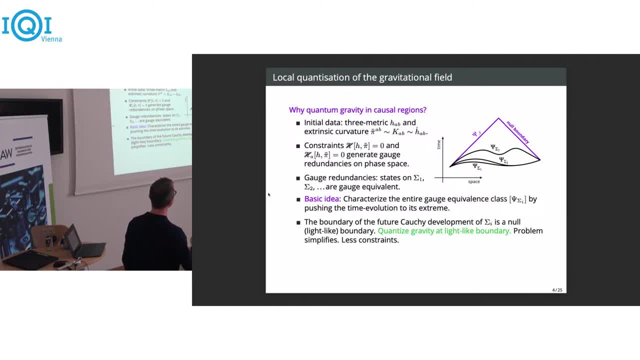 And so these states, let's say classical states, on different Cauchy surfaces that are related by the hyper surface deformations, They define the same Physical state, and imposing these constraints is very difficult in quantum gravity, or the problem of quantum gravity is to make to make sense of the solution of this constraints or to make sense of quantizing these constraints. 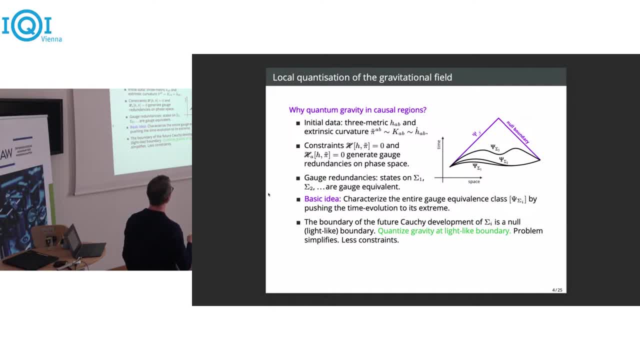 But what this means intuitively is that so these different states are gauge equivalent, so we can, and the gauge equivalent data is Is hard to analyze, So patterizes these gauge equivalent class. So one way to characterize these gauge equivalent class is to push this evolution to its natural extreme. 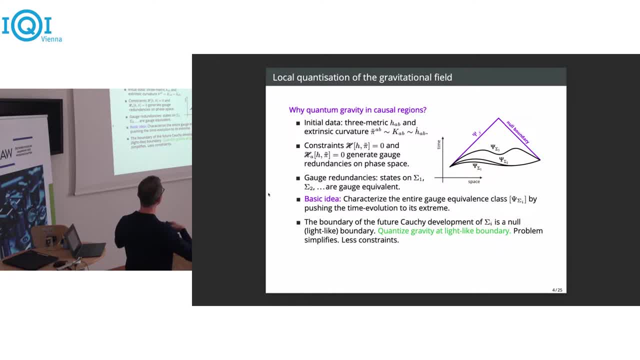 namely when it hits The boundary of the futureui development Of this partialck she's surface, and this is an. So, instead of trying to imposing or solving at the quantum level these constraints that imposed the village认ي ble It stands for exist. 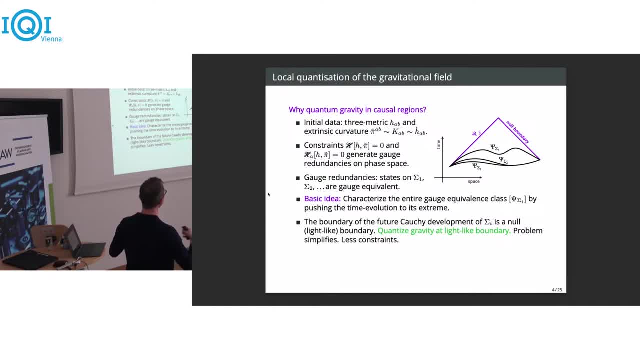 we can take now a different viewpoint where we characterize this gauge-equivalent class of initial data. so different solutions or configurations of extrinsic curvature and three metrics. that satisfies the constraints, but different such solutions are gauge-equivalent. How do we characterize this complicated gauge-equivalence class? 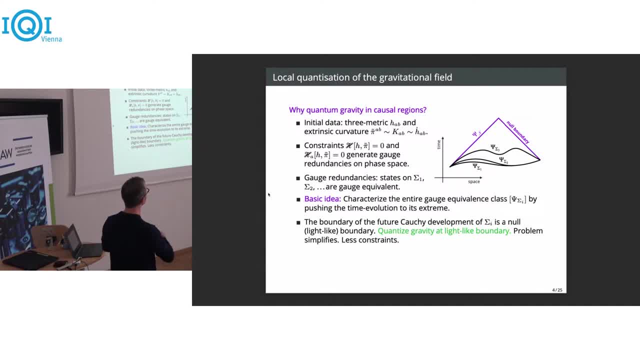 Well, one way is to go to the null boundary, to the boundary of the future Cauchy development of these slices. Then the idea is to quantize gravity there, so to quantize the initial data on these null hypersurfaces. And the problem now simplifies. 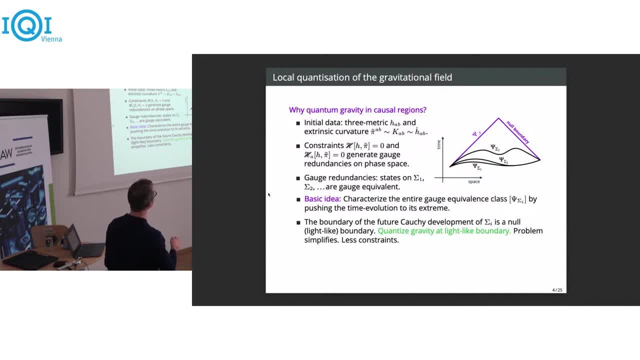 because now we have to quantize less constraints than before It happens. It happens so that we don't have to evolve anymore back into the bulk, so to say, because the data at the null boundary already characterizes this entire gauge-equivalent class. 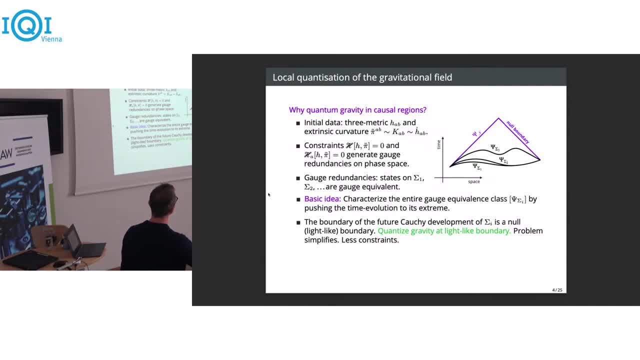 So we are left with less constraints, In fact only the fumorphisms that preserve this null hypersurface, And in that way the problem simplifies. Yes, This is good Point to ask conceptual questions, But then you have to give a prescription: what sigma 3 should be. 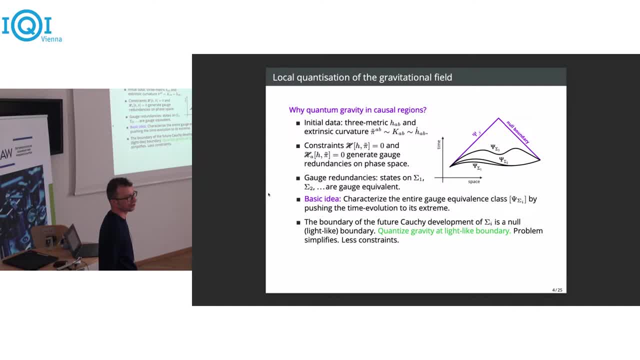 For instance, it could be a surface of constant mean curvature or a surface where the trace of the extrinsic curvature vanishes. So this is also a viewpoint which is being investigated, in fact, Like the conformal method of solving the constraints. But my viewpoint is that 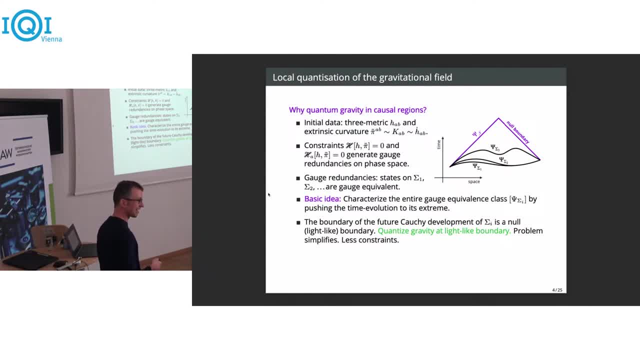 and this seems to be supported by the evidence- that, then, the problem is still as complicated as before, While at this the point is that at the null boundary, there's just way more structure available that we can use and that we should take advantage of. 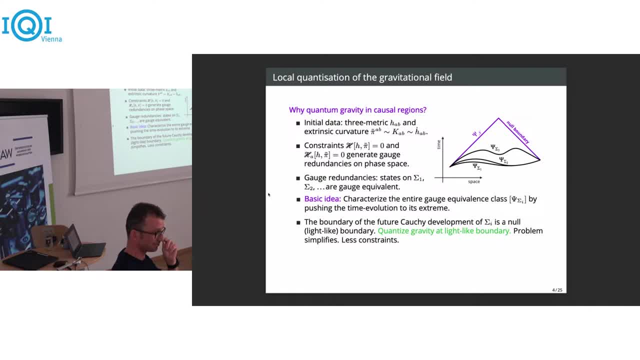 Yes, Just another question. In your picture you have the surfaces that are especially compact, right? They're not exactly Gauchy surfaces: Mm-hmm, mm-hmm, Extend to infinity, and then they actually have a boundary. 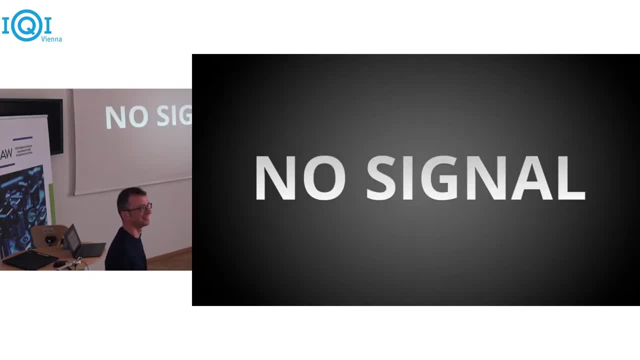 That's right In your case, if you take into account true Gauchy surfaces. what do you do? Do you do it on like or something? So this is a very good, really very good point The view, but now my screen, I cannot answer it. 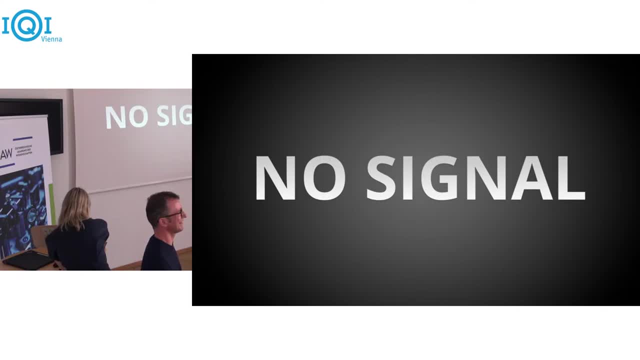 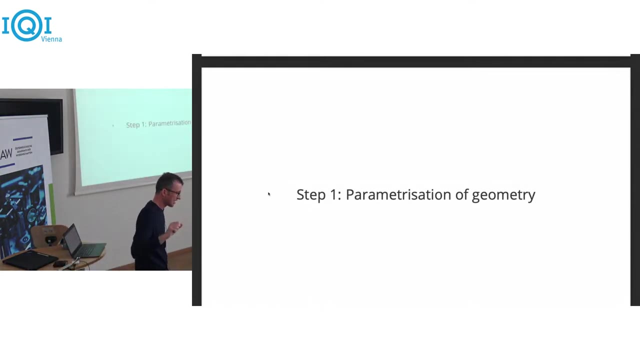 Like this. So the usually people would do precisely this. They would go to null infinity and quantize the geometry there. The problem with this viewpoint, in my opinion, is that there are now two limits that may no longer commute. There's a limit where or you can first say: 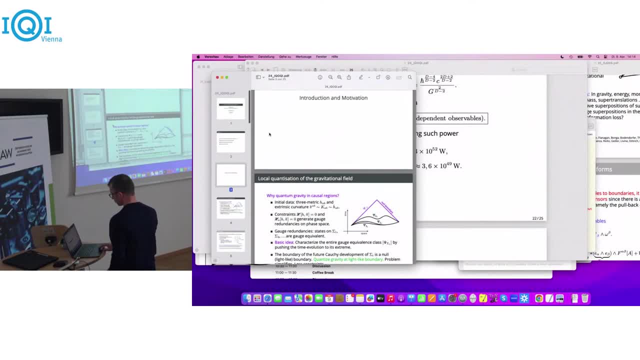 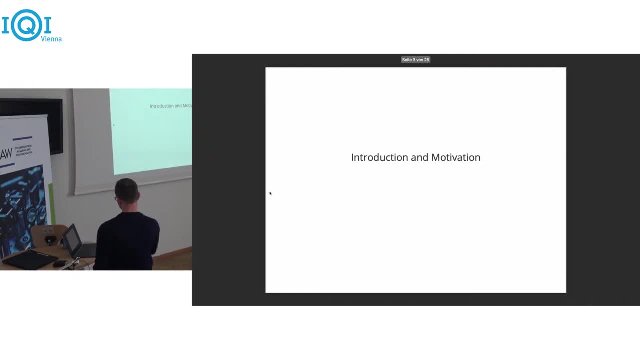 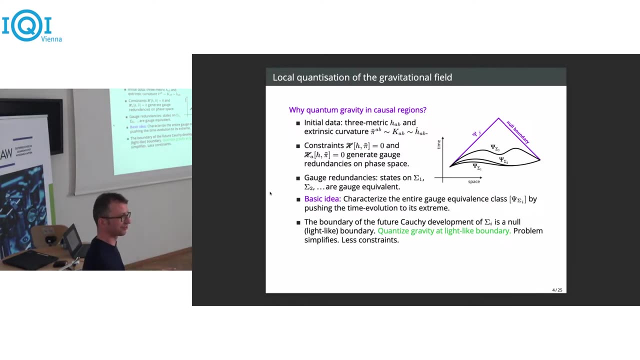 let's start out with the geometry. let's first start out with partial Cauchy hypersurface, Define the phase space there and quantize it, And then, within the quantum theory, take the limit to infinity, to null infinity. 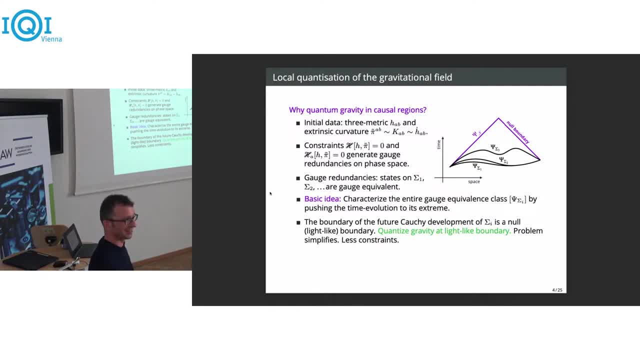 But that may not commute with first taking the limit to null infinity and then quantizing- And this may be in fact related to some kind of you know- But that may not commute with first taking the limit to null infinity and then quantizing. 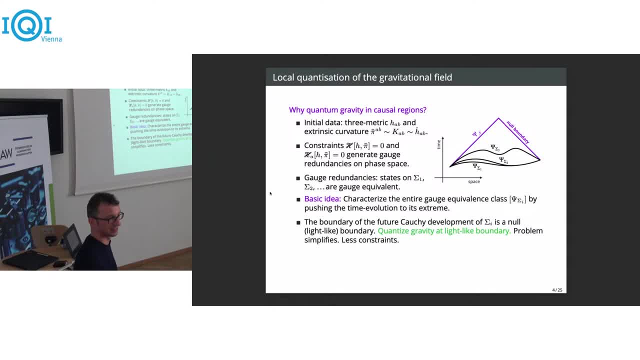 And this may be in fact, related to some kind of, you know, certain infrared ambiguities. I believe in quantum gravity that appear in the s matrix approach. so there are two limits, and what I'm saying is it is possible to make sense of quantizing gravity in finite regions. 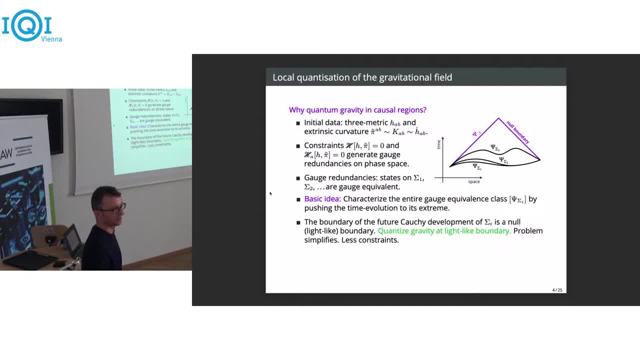 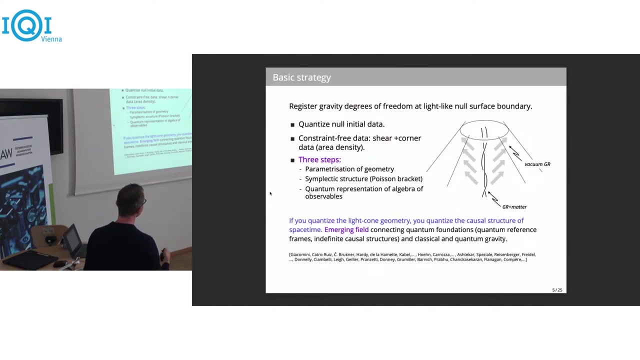 I. so I consider the initial data on the null boundary, and then there will be a phase space, and the phase space can be quantized. but I will outline this step by step. so, in fact, this is precisely the viewpoint. we, instead of dealing with the, call a complicated system. 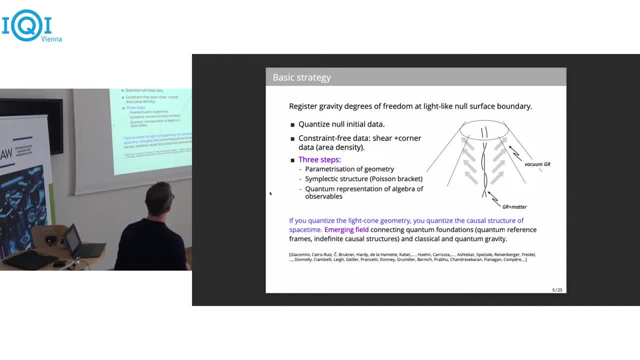 of, for instance, an inspirer of two black holes that can then emit gravitational waves, be and and. to study that one would have to look at the spatial cushy hypersurface. the viewpoint is we look at physics away from the source, where we register null initial data at a null surface that can, where 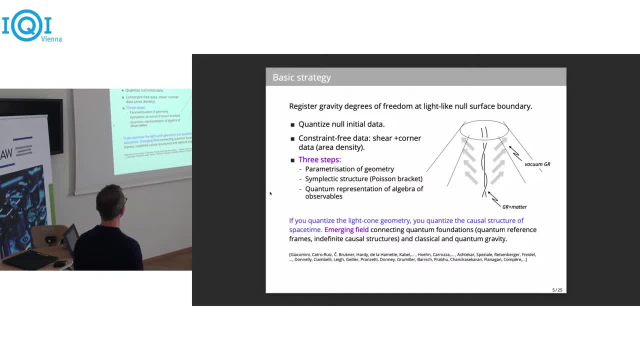 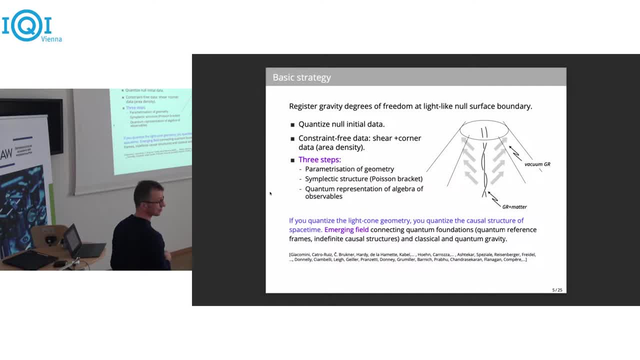 parametrization of the geometric data at the null surface. then you need to equip this space, this space of geometries, with the symplectic structure that did inherit from classical general relativity, And then you have to find a quantum representation of the algebra of observables. 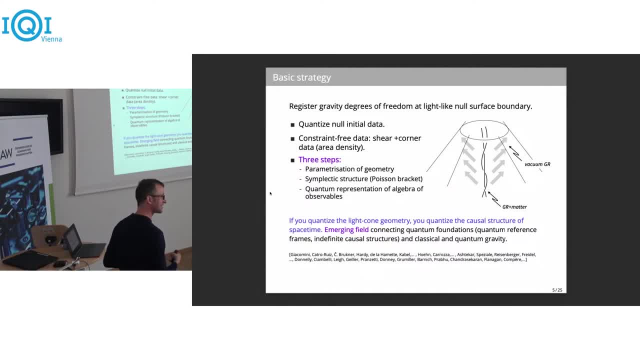 And what is really exciting is that this seems to bring together really different approaches. And I can speak here at the Institute of Quantum Optics and Quantum Information because there's a lot of interest in quantum reference frames, indefinite causal structures, But I could equally well have given this talk. 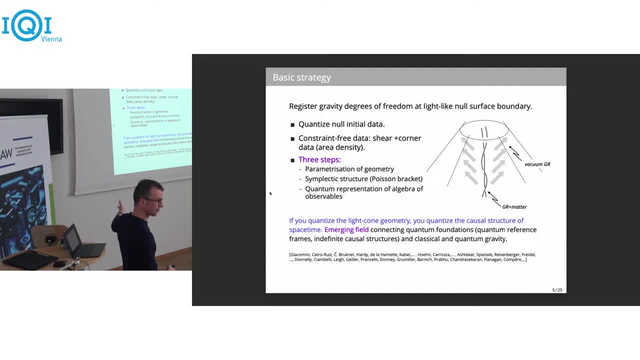 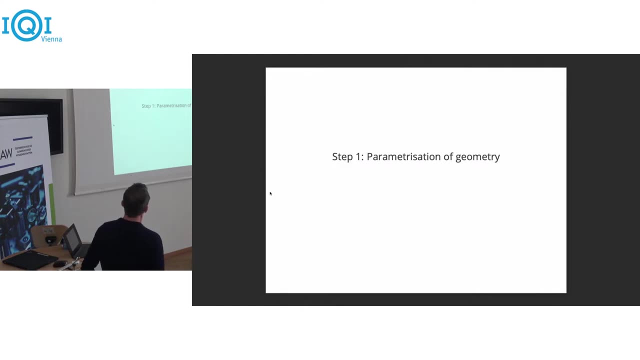 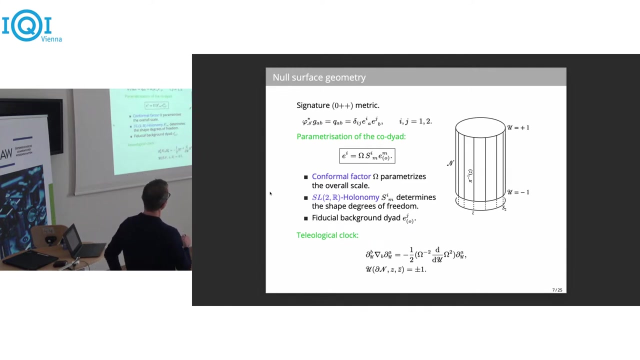 In fact at a conference that is just being organized close by at the Erwin Schrödinger Institute. So there's really something happening that different communities come closer together, which is exciting. Step one is to find a parametrization of the geometry. 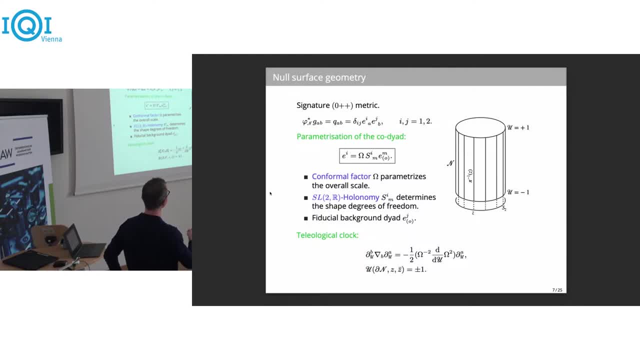 In here. topologically, the null cone- ignoring caustics for a moment- is just a cylinder, And in fact I consider only an interval of the null surface. So what I'm interested in is to assign a phase space to a null boundary, but only to a portion of a null boundary. 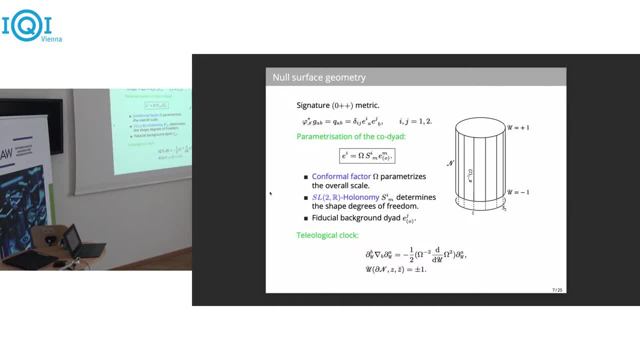 that will actually extend. And then the basic strategy. If I can make sense of the phase, space and quantum geometry of one such strip, by gluing quantum states together I can actually build an entire light cone geometry. So the first step is to just look at one such band of nulls. 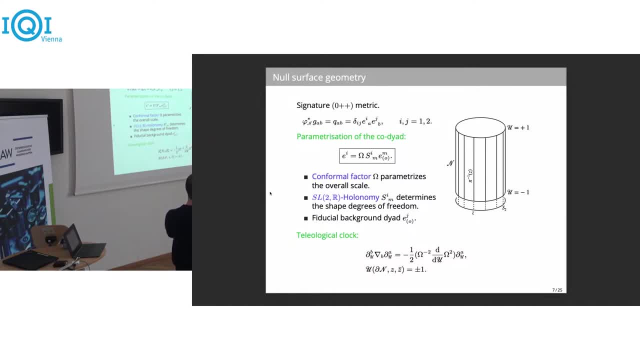 at the portion of the null boundary that is itself bounded by two cuts, The initial cut and the final cut, And now the geometry. now, this is a null surface And relativists we all know, in relativity this null surface boundary is generated by light rays. 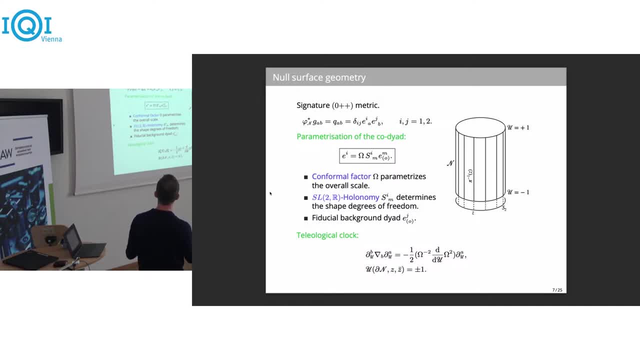 And then the geometry is determined by the metric. And if we take the pullback of the spacetime metric to the null boundary, we get an intrinsic metric tensor on this three-dimensional manifold. But this is a very complex problem. It's a degenerate metric. 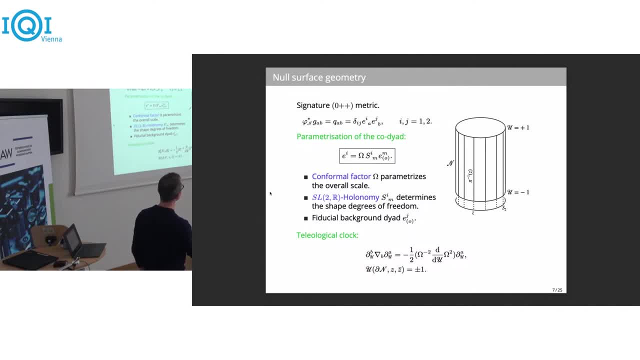 So it has a one degenerate null direction, which is of course the direction of the null rays themselves. Diagonalize this metric tensor And since the geometry is two-dimensional but there's one degenerate null direction, I only need two autonormal frames, two directions. 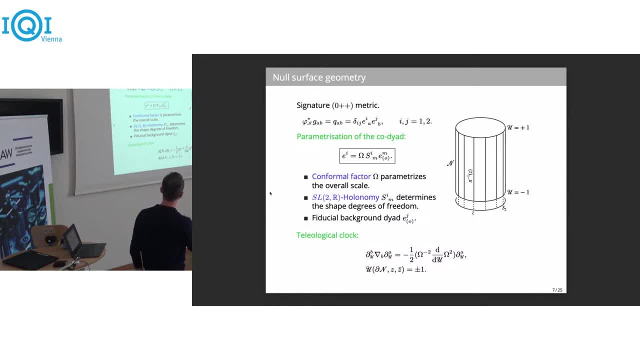 two co-diad, so basically a co-diad. And then I have to do this, And now any such co-diad can be parametrized in the following way: We introduce an overall scale, a conformal factor, And then there are the shape degrees of freedom. 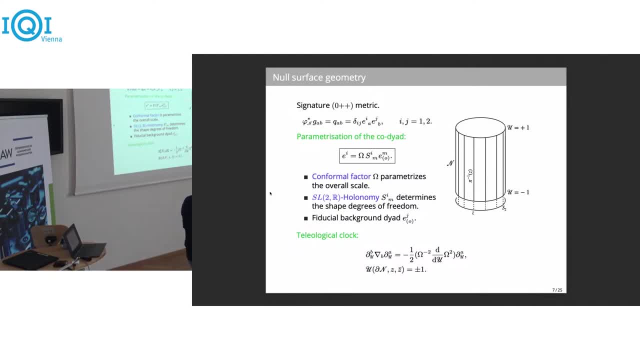 that are encoded into an overall SL2R holonomy. Pictorially, you can think what's going on here as follows: The geometry, The, The null directions have zero length. There's no geometry along these generators. The entire metric is basically two-dimensional. 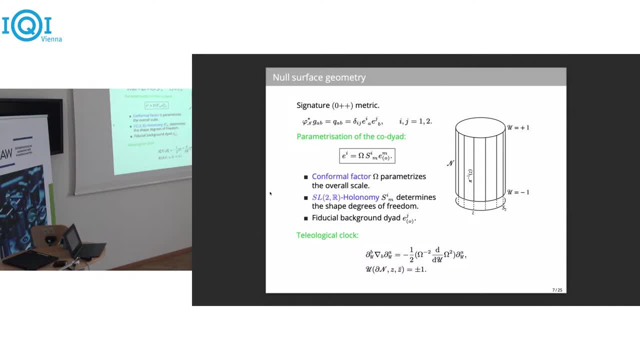 with one degenerate direction. Now, a two-dimensional metric determines the shape of triangles. let's say No. And so, to understand the degrees of freedom in this metric or in these autonormal frames, we can think of these triangles. Now, the triangle will be characterized. 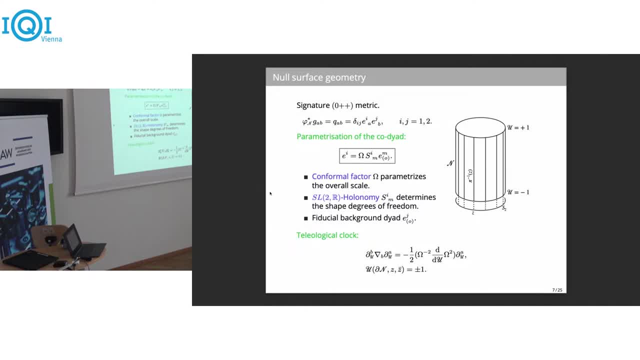 by its overall area, which is encoded in the conformal factor omega, but also in shape. degrees of freedom. They tell you that, however, preserve the area. So these triangles should all have the same area, but different shapes. And going from here to there, you have an SL2R. 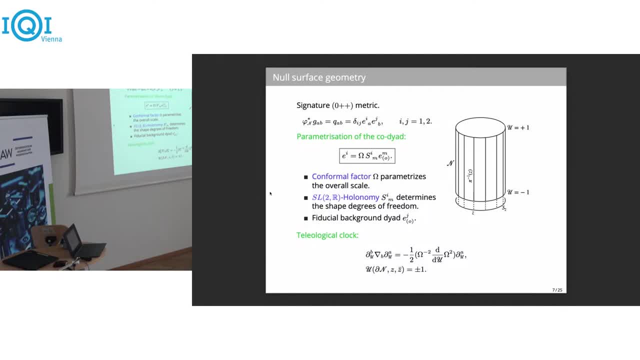 And going down, you have a conformal factor. This encodes the geometry. This way we can encode the geometry of the null cone by an overall conformal factor, omega, and an SL2R parallel transport. In fact, I call this holonomy or parallel transport, because 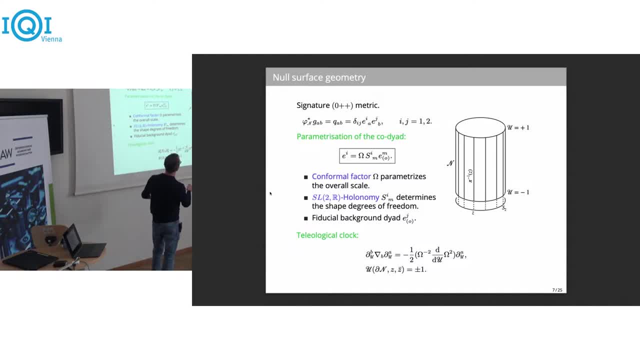 this matrix is parallel. does in fact tell you how to parallel transport along this light rays And this 0EM0,? this is just a fiducial reference frame, Fiducial if we think of the geometry of this null boundary as S2 cross R. 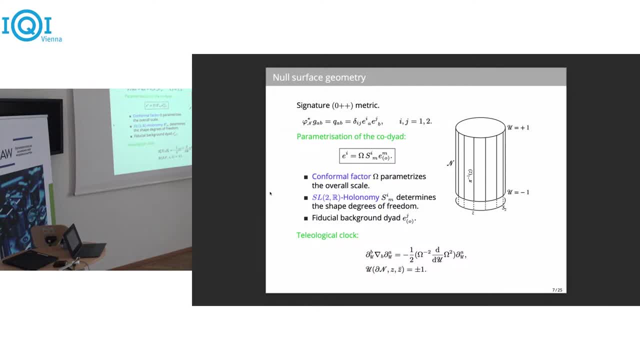 so you take S2 and you shine light out of this null surface, then this possible choice for this fiducial reference frame is just: E1 is d theta and E2, 0, sine theta d phi, So a round metric on the 2-sphere. 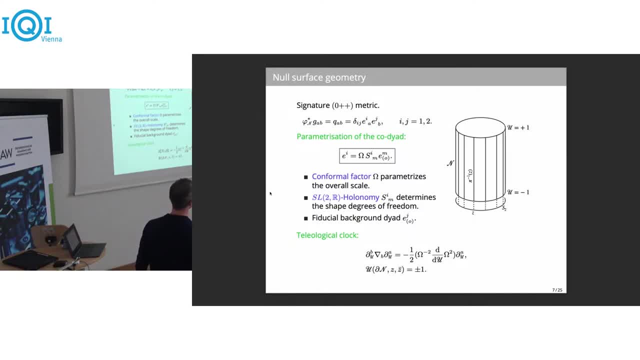 Okay, But determining a round metric, which would determine a round metric at the 2-sphere, but the physical metric is expressed relative to this reference, flat, round reference metric. But on top of that we need to choose, or what I want to choose is a choice of clock. 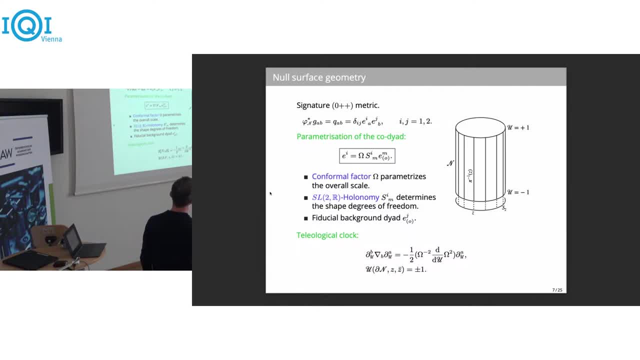 a notion of time along this null rays And there is no preferred choice available. You can choose whatever you like And for reasons that become more obvious later on, the following choice is useful Where what you have here is the. if on the right-hand side, you would have 0,. 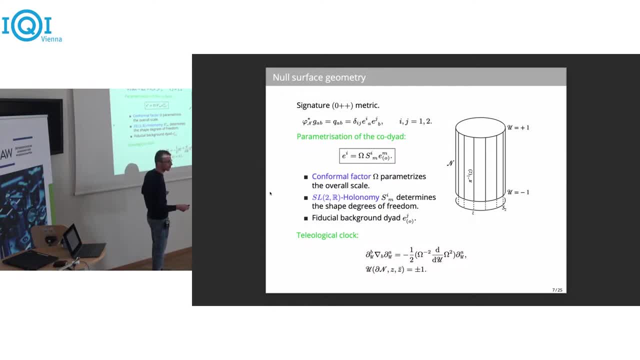 this is what we call an affine parameter. This is the analog of proper time along the null rays, But I correct this by a term that is proportional to the expansion of the null rays. So this is a measure for how the area of this geometry 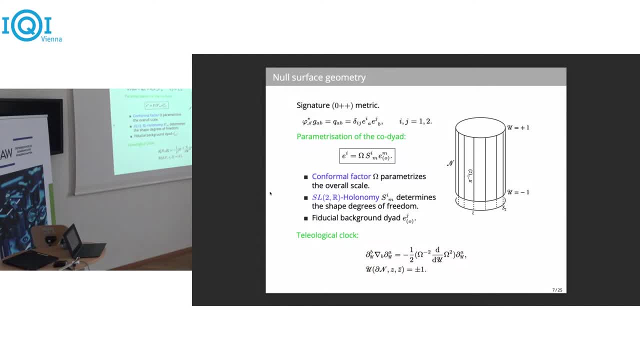 the area. density changes as we move forward in time And, furthermore, this clock I choose such that the initial and final cross-section, the initial and final cut, have just values plus, minus, And this choice is always available. Now, this describes the geometry. 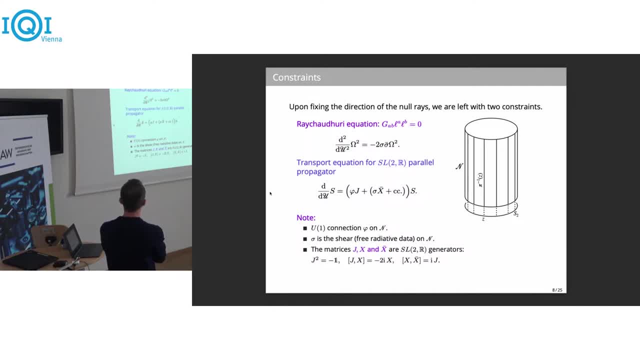 a generic geometry of a null hypersurface. But now, not any general geometry is consistent also with the Einstein equations. To impose the Einstein equations at the null boundary, for the null boundary geometry to be consistent with the Einstein equations, you have to impose the Raychaud array. 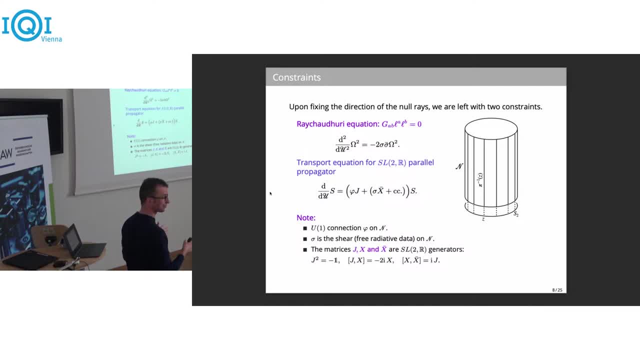 The Raychaud array is the same as the Einstein equation And nothing else, which means you only have to deal with this one constraint. In addition to that, there is a- well, there is also a transport equation for this SL2R holonomy. 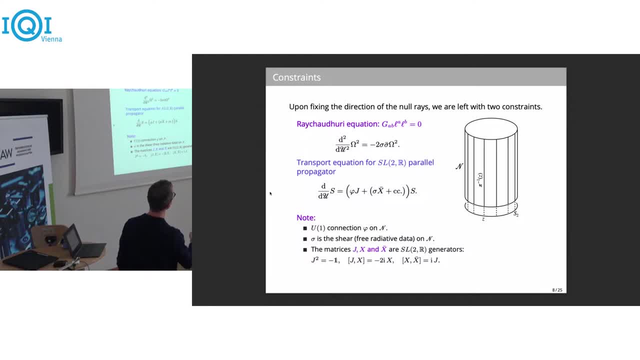 along this SL2R parallel transport, along the null generators where sigma is now the shear. If, if this, if the shape of these triangles is conserved along the null generators, the shear is zero. if the shape of the of these triangles changes as. 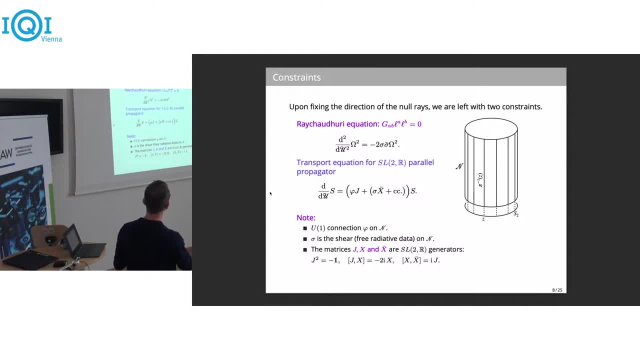 we move forward in time, the shear will not be zero, will be non-zero, and it will encode. in fact- and in fact this is the effect of what gravitational radiation does- is, if gravitational radiation crosses the null boundary, it will affect the geometry by, by changing the, the. 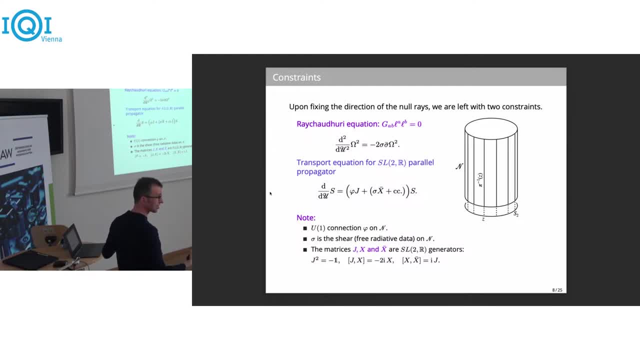 shear degrees of freedom, so gravitational waves to this shearing. yes, this is on top of that. so for the right, sure, a really equation, the in the right shadow we equate the right short right. chowdhury equation with respect to this clock turns into this simple second order differential equation for the. 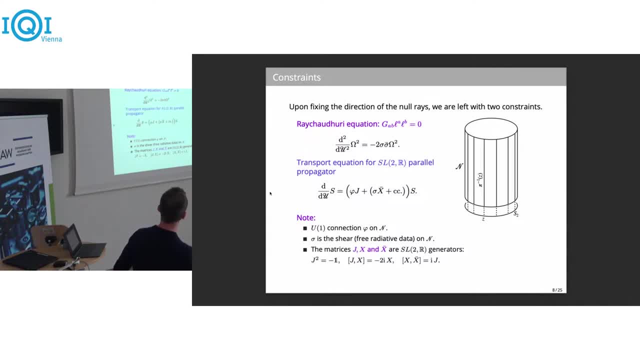 conformal factor which is sourced by the shear degrees of freedom. and the shear degrees of freedom you read off by solving this equation or by taking the time derivative of this SL to our holonomy. this defines the shear degrees of freedom, and then you insert the shear into. 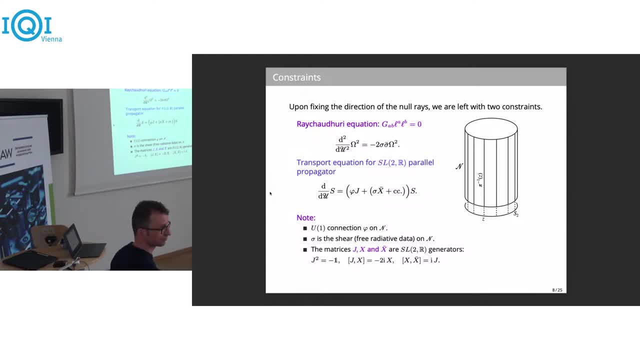 this equation to solve it for the conformal factor. yeah, yeah, this is this just the definition of the shear the, the shear degrees of freedom that enter the right shadow equation derived from first derivatives of the metric, but the metric is now encoded into this SL to our holonomy. this is why first derivatives of the SL to our holonomy. 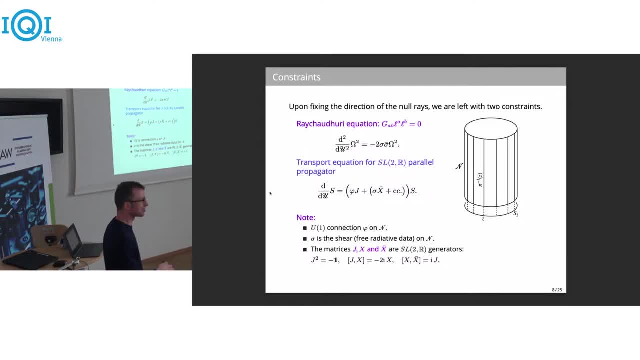 define the shear degrees of freedom, and then you insert the shear degrees of freedom and then you here. It's just a change of variables, precisely. So the question is how to translate the original geometry into this SL2R and conformal factor. So this defines the geometry. This gives you. 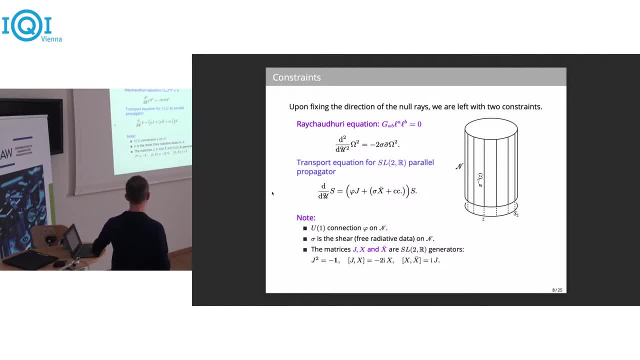 the geometry in terms of the variables chosen, And it is not arbitrary. It has to satisfy certain constraints And the constraints are given here. And notice that there is also U1.. This is just because we have, by going to autonomous frames, we have enlarged, we 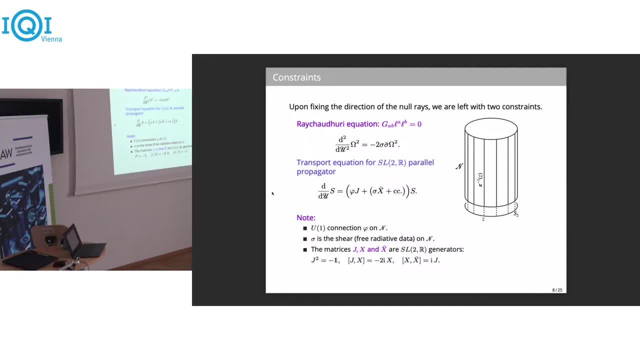 have a further gauge, redundancy, which is basically, which is nothing else than a rotation in the plane of this. It's triangles, intuitively. So there's also U1.. So there's a U1: degrees of freedom that rotate your frame fields. Then there's an SL2R that encodes the shape: degrees of freedom. 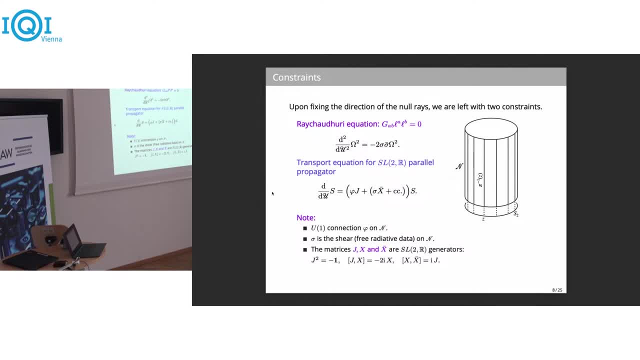 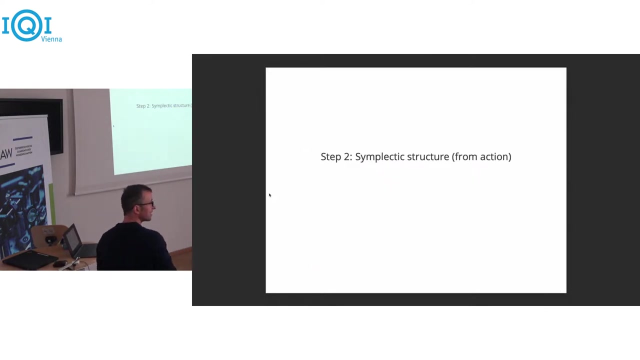 And then there's a conformal factor that determines the size of the metric at the null boundary, the overall scale. And so phi and sigma are fields on the null boundary, And J, X and X bar are matrices, just the generators of SL2R. But it's not enough. structure phase space algebra of. 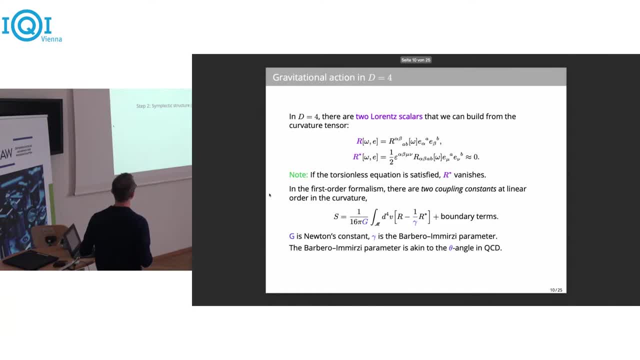 observables to then speak about quantum theory, And so we need. the symplectic structure derives from the action. The action I use is just the usual GR action, with a slight modification, a modification that does not change the equations of motion, but it affects the symplectic structure. 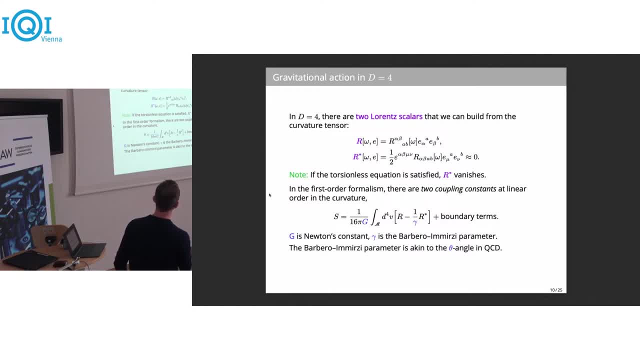 And this appears only in D- equal 4 spacetime dimensions, because in D equal 4 spacetime dimensions in the first order formalism, when you work with tetrads and connections, you have two curvature scales. So you have two scalars from which you can build an action that is linear in the curvature. 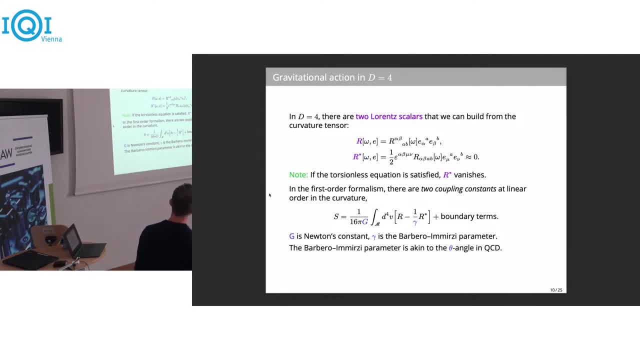 And this action gives you back to Einstein equations. And this additional coupling constant that now appears is akin, similar to the theta angle that appears in QCD And at the quantum, at the classical level. this has no consequences at all, It just changes. 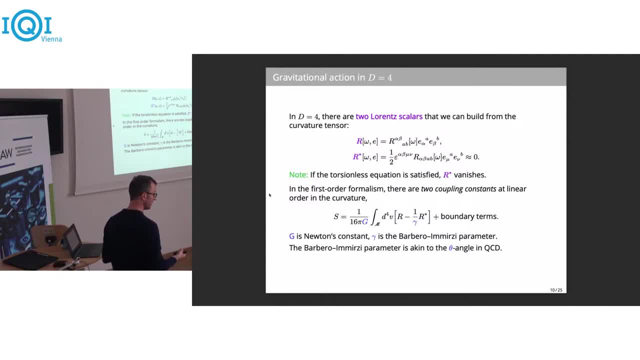 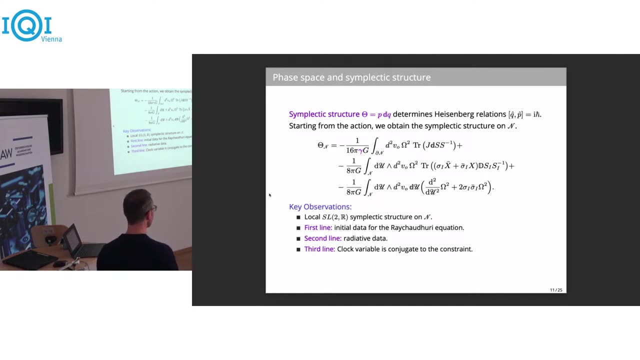 the way you think about phase space. It does not change your the solutions to your field equations, but it does have effect. effect in quantum theory And we will see how this will play out. in fact, And from the action you can define the symplectic structure And then you obtain a symplectic. 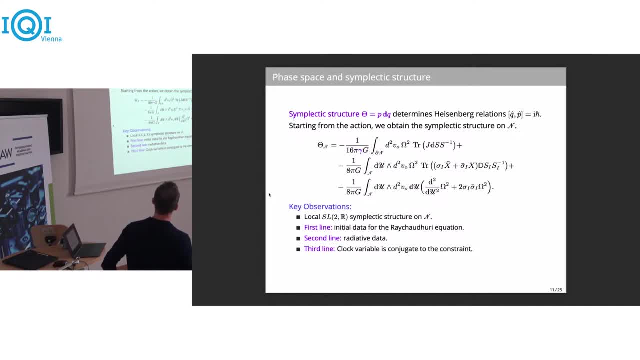 and the symplectic structure in. well, in mechanics this is just P, D, Q. This D is this bold D symbols. These are uh uh differentials in phase space, To distinguish them from differentials in on the manifold. 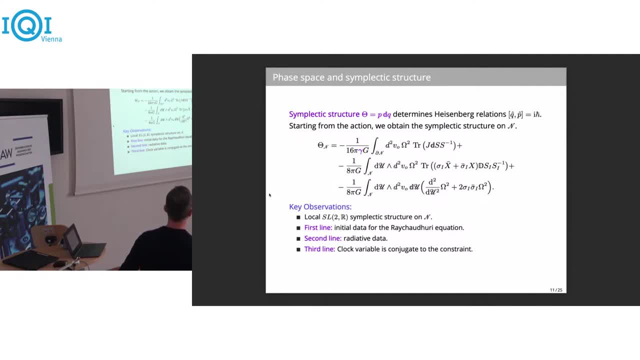 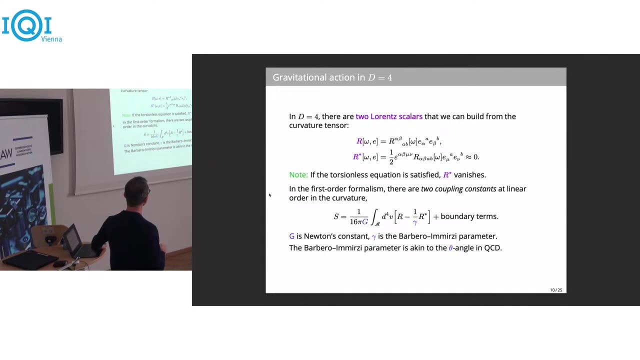 That's what, uh other authors would just write delta for variation. What is important here is that the symplectic structure. we need it because this gives us, at the quantum level, the algebra of observables And starting from the action we chose. so this uh, gamma action that contains the so-called 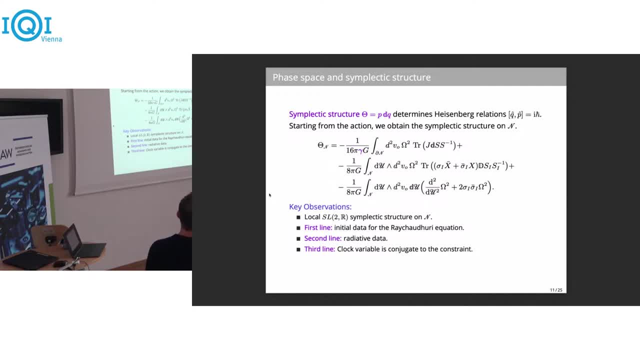 Barberon, emersibility, The Merce parameter. we obtained the symplectic structure on this null strip And this has now three terms. What are these three terms? Well, first of all, we observe that this is basically an- uh um, symplectic structure. 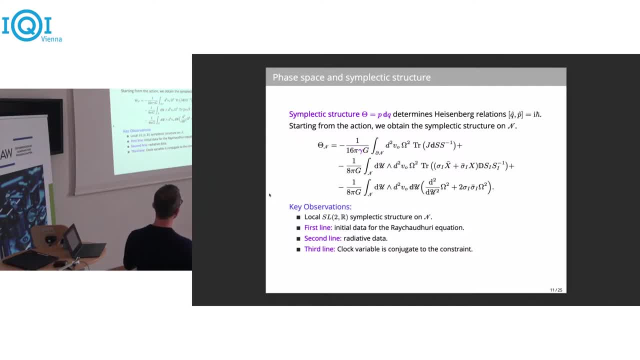 for SL2R matrices group. elements that, however, depend on that are fields on the null boundary, that are fields on N, And what we also notice is that there are different contributions, contributions- there's one contribution coming from the boundary, from the cuts. 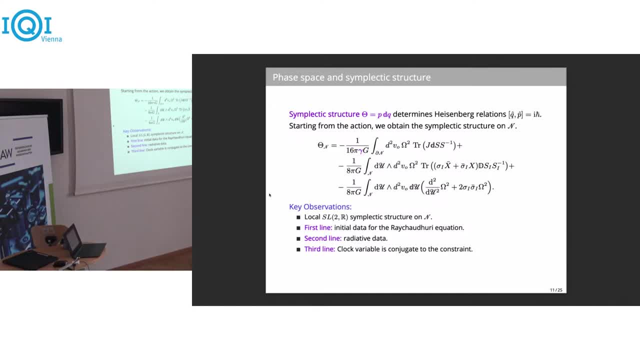 from the two cross sections that I introduced- the initial cut of the null boundary and the final cut of the null boundary- and what we see here is that you one part of the SL2R is canonically conjugate to the area density. and then there's the second line. these are somehow bulk degrees of freedom, or 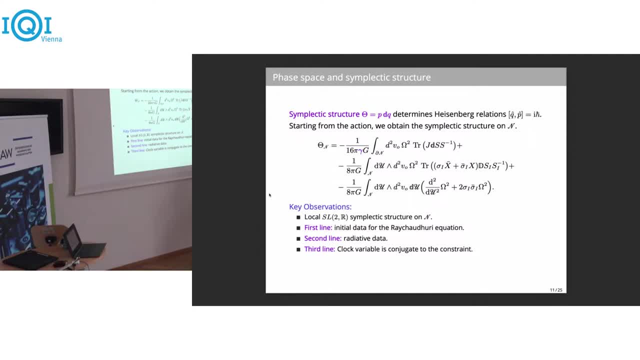 degrees of freedom that live along the null hyper surface. these are the radiative modes. and these are precisely these shear degrees of freedom. don't wonder about this subindex I. I will come to that in a moment. it's not that important. so the second line encodes the shear degrees of freedom, the this SL2R. 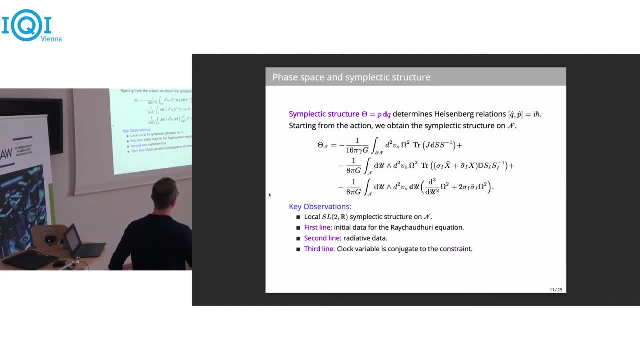 matrix is canonically conjugate to a SL2R Lie algebra element, and the third line is the clock. so the clock, the time variable that we introduced, is canonically conjugate on phase space to the constraint. this is not so surprising. the constraint, after all, generates gauge. 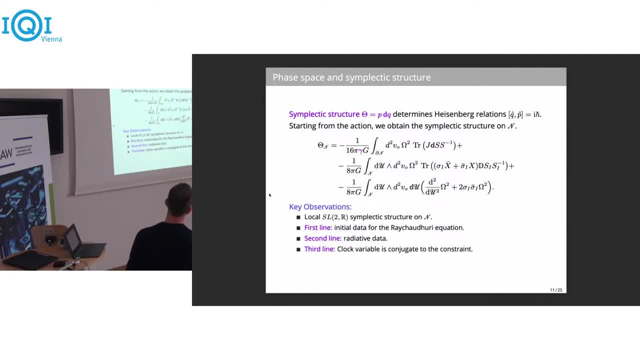 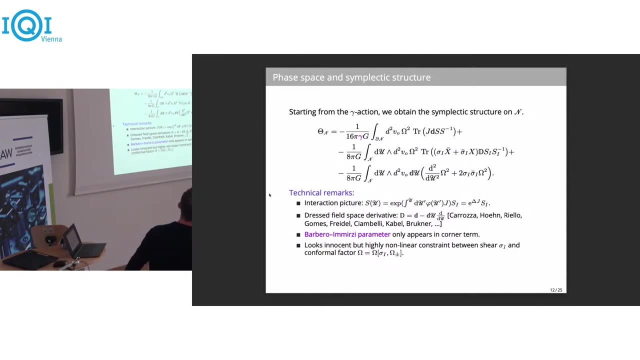 symmetries. the gauge parameter is the time variable, so the at the Hamiltonian is the time variable, so the at the Hamiltonian is the time variable, so the at the Hamiltonian level. the constraint generates shifts in the time variable. a few more technical remarks. so I introduced this index I here. this is just a kind of u1. 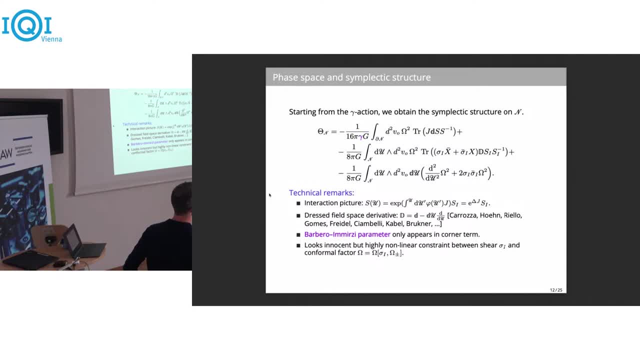 interaction picture where I split off this, you one factor into into a dressing of this shear degrees of freedom and this capital D here is addressed. field space derivative: it is the ordinary variable variation minus a diffeomorphism, but only a diffeomorphism along the null. 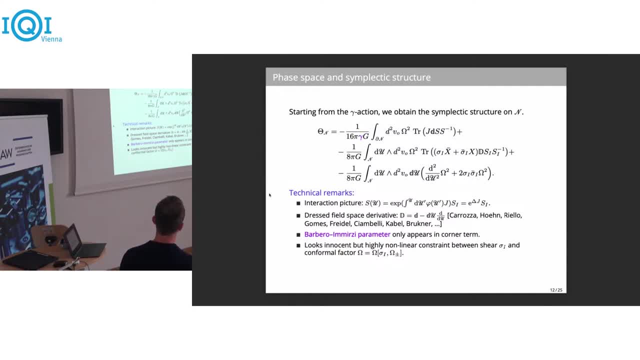 race. So changing the clock, And also note that the Barbero-Emmers, this additional parameter, appears only in the Kroner term and this is very typical to terms that you add, or this is typical to terms in the action that you can add. but 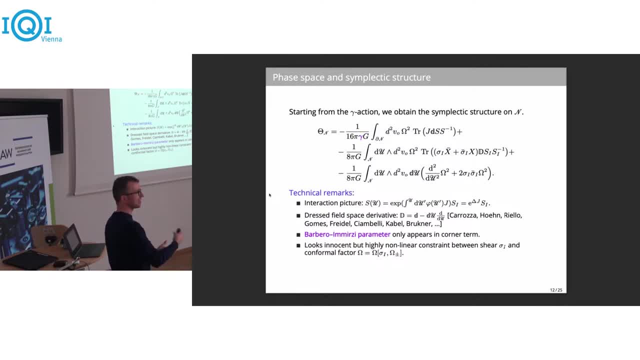 do not change the field equations. They only generate terms, Kroner terms, that change Eosimplectic structure but do not change the field equations. The whole thing looks very innocent in a way, but this is remember that this is now highly nonlinear because there's a constraint. The constraint says that this: 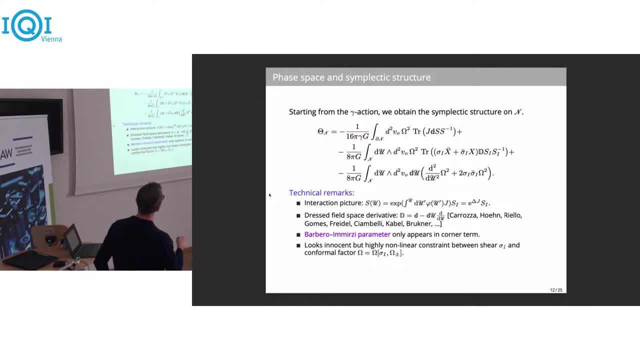 term in the bracket vanishes. so you have to first solve this omega. so even sigma, sigma bar as free data, you can solve this equation and then plug it in into the second line. okay, so omega will depend in a non-linear, highly non-linear way on the shear degrees of freedom and on. 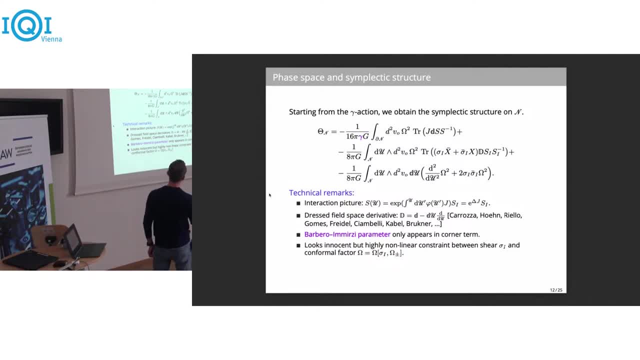 additional initial data that you have to specify. the reichardt equation is in this. with respect to this clock, it is a second order differential equation sourced by the shear degrees of freedom, a second order differential equation for the conformal factor. so to solve this equation, you 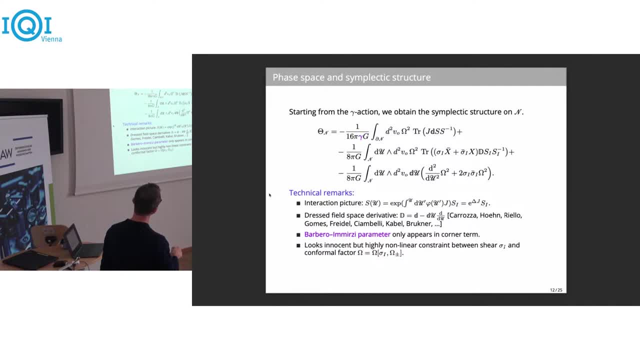 have i, you have to give me the shear as three initial data along the null boundary, but you also have to give me initial data for omega. two initial data, either omega and omega dot, or just omega at the two cross sections. but these cross sections the initial data for omega. 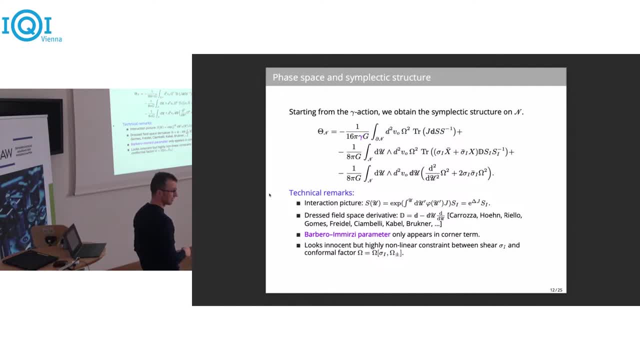 has now its own symplectic structure, which is good. this means that at the quantum level, everything becomes quantum. the shear degrees of freedom become quantum because there is a symplectic structure for them, but the corner data, the data at the cuts, that determines the initial. 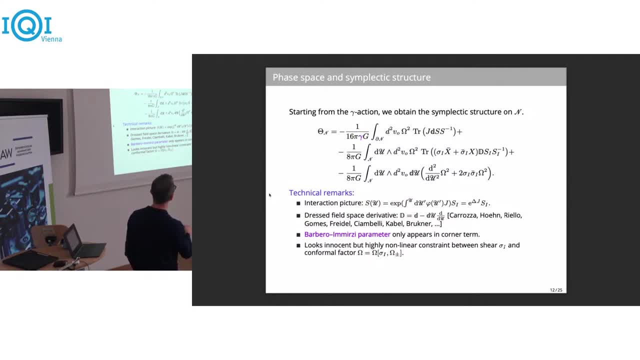 data at the two cross sections for solving the reichardt equation will also have its symplectic structure, so it can also be quantum and this is something that is can never be seen in the asymptotic quantization, because in what happens asymptotically, if you go to scry, if you go to scry. 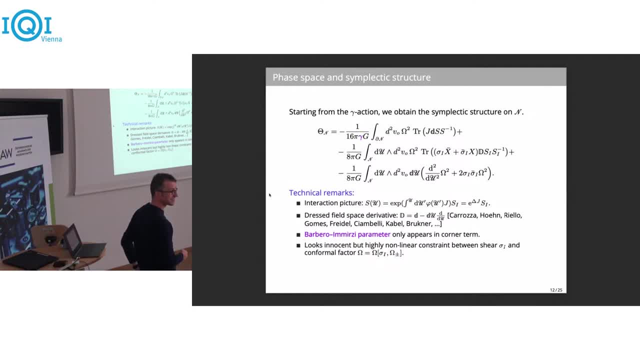 we send, what do we? what happens? we send the area to infinity. obviously we go to infinite distance from the source. so this, this uh, two, two surface cuts these two dimensional spheres, let's say they become infinitely large, they become the celestial sphere. in fact, that's why people 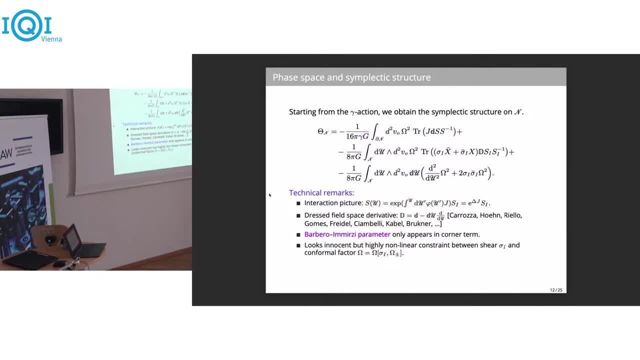 speak about celestial holography. but the celestial sphere has infinite area, it's. it is an infinite distance, but this is of course an approximation. we do not make observations at infinite distance from the source in any realistic experiment. we are at finite distance. in fact. scry may not even appear. 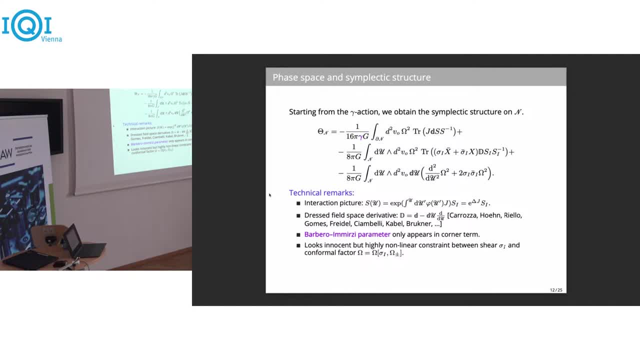 in any realistic experiment. we are at infinite distance. in fact, scry may not even appear for generic initial data or in when we are in in a situation with a positive cosmological constant. there is no asymptotic boundary which is light like. but all this still holds, so that that is why 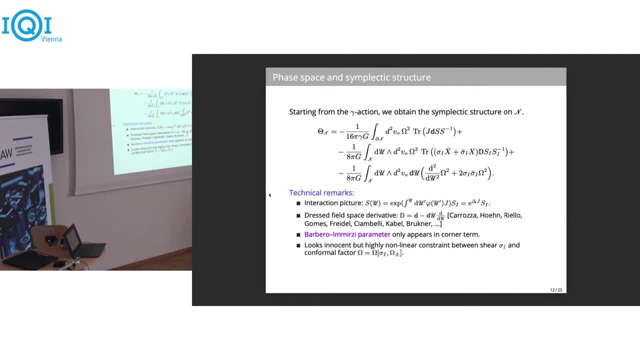 this is also interesting and um yeah. so what happens if we go to an asymptotic boundary? then we would send this observable at the classical level to infinity. but this is in conflict with the heisenberg principle that you cannot send a classical quantity just naively to infinity before. 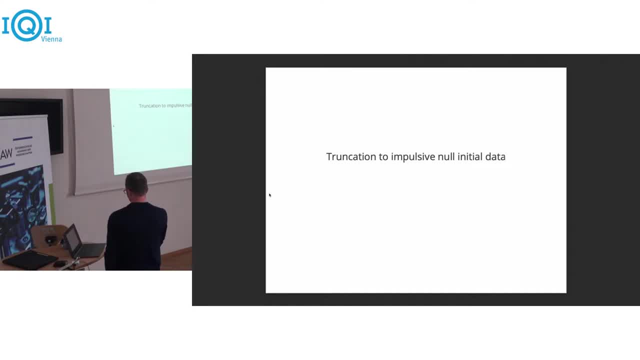 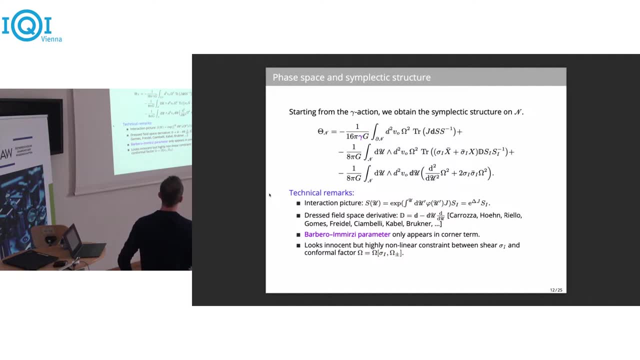 going to the quantum level. but now all of this is highly complicated, i said, or highly non-linear, because omega depends on the shear and the initial data in a in a complicated way because you have to solve this second order differential equation for arbitrary shear. so this seems, uh, and then 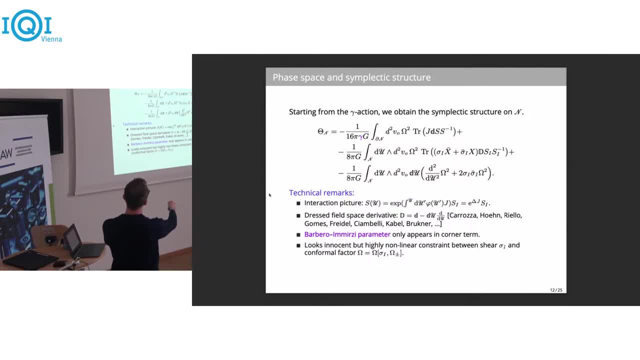 it appears in here, and inverting the out of the symplectic potential. you have to compute the symplectic two form, invert it and then find a quantum representation. but this is very difficult because everything is now non-linear. all the non-linearity of general relativity is now in here. 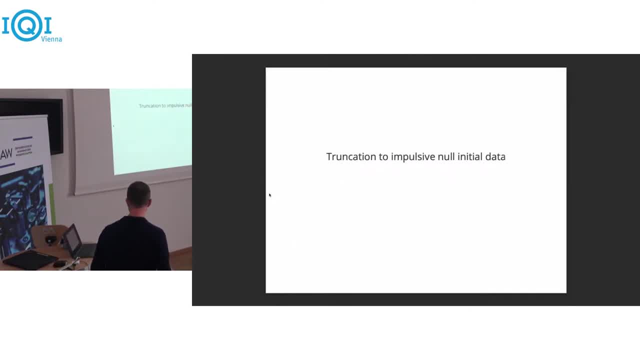 but there is perhaps a way to do this systematically in the following way. so what we can do is simply to restrict ourselves to a specific class of null initial data, namely those where the profile of the free initial data follows the follows the shape of a step function. 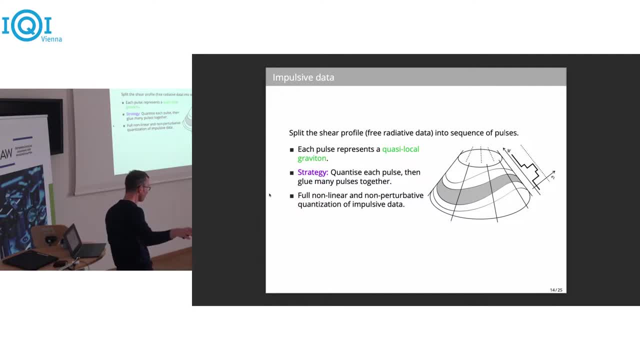 and we know that any smooth, smooth function can be approximated to arbitrary precision by just very tiny, uh, very short such step functions that we can use in this particular stud in the original method. so we have a good idea about so. if you have a little more time to ah, think about this problem, it's just a way to learn lectures. 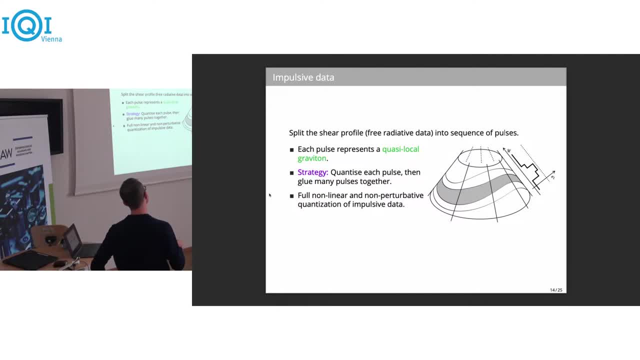 about the function of the flow in the original method. so what we can do is just to look at the function of the flow and we can also let you know the terms of the flow in the original method. so, for example, if we have r with the r of z, weigh r with r of t, and then we just call this r of t. 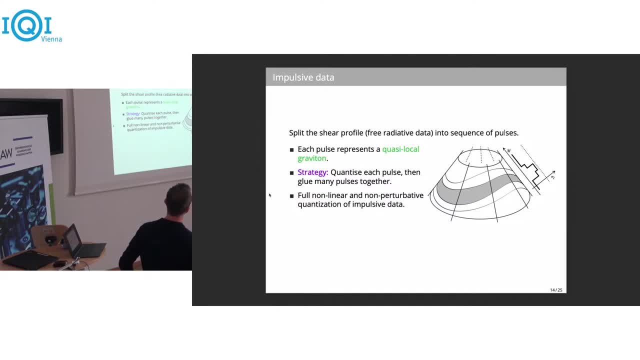 a more general profile, we would take the tensor product of many such Hilbert spaces and trace over the intermediate boundary modes or edge modes, And in this way, I claim, one can construct a full, non-linear and non-perturbative quantization of gravity on the null cone. So far, 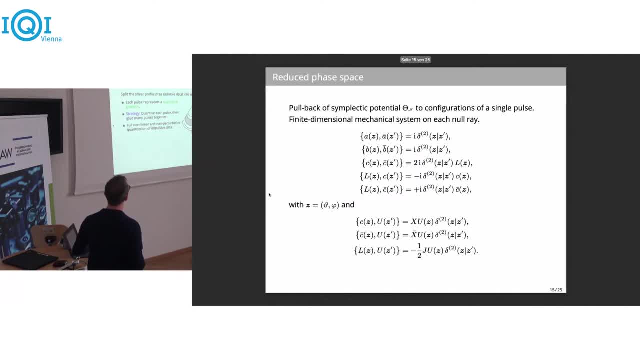 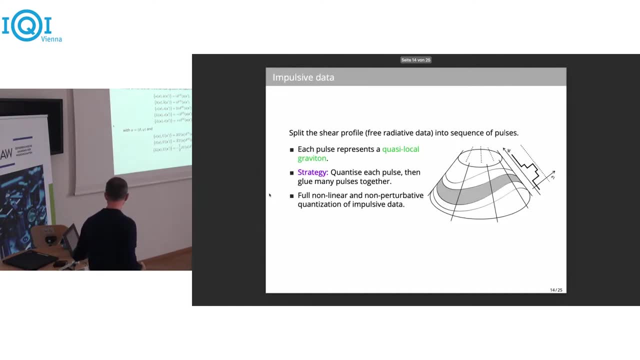 I'm only looking at the single parts, But now of course everything is simplified, because now the pulse is only characterized no longer by infinitely many degrees of freedom, but only by finitely many degrees of freedom, namely the height of this, just by numbers. 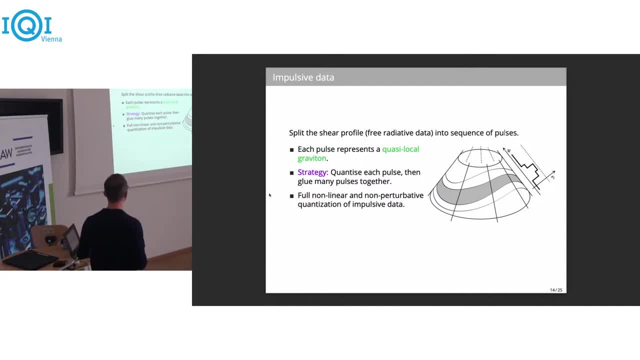 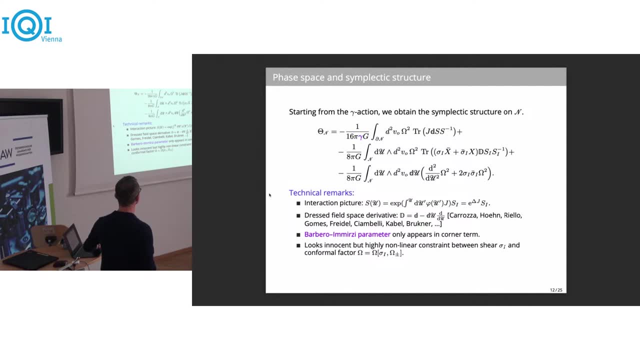 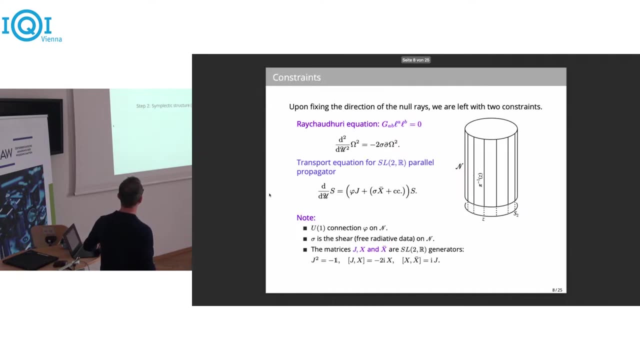 not fields the height of this pulse. And if you now, if you- and now the point is actually sorry for jumping back- If you, What I now introduce is truncation, namely I restrict myself to configurations where the shear is constant, piecewise constant, But then this equation becomes simple. 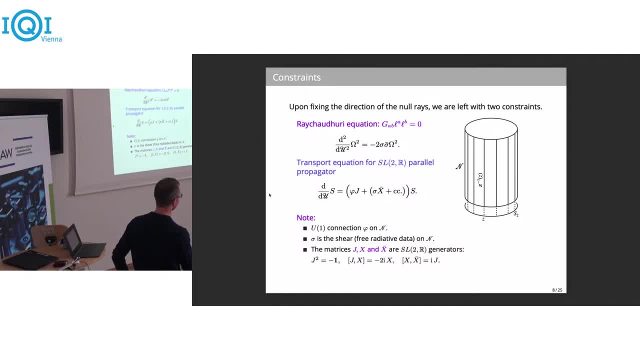 This is just a simple second order differential equation with constant frequency. No, everyone can solve this, and here here also. so if sigma has the u1 part, you can split off and then the shear is piecewise constant. if the shear is not piecewise constant, 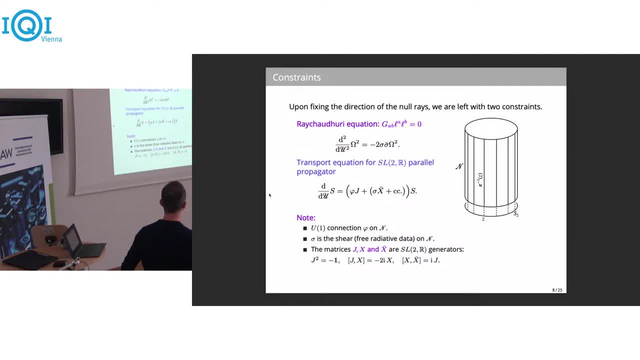 you solve this equation by a part time ordered, exponential in u. this is like a Schrodinger equation with a Hamiltonian that is in general time dependent. but if so you need a time ordered product. but if sigma is just constant, you can solve this immediately. constant with respect to u. 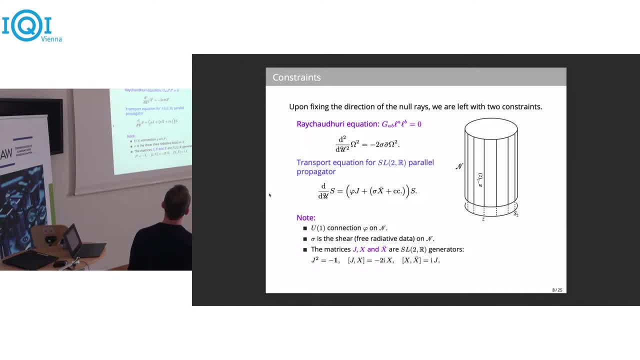 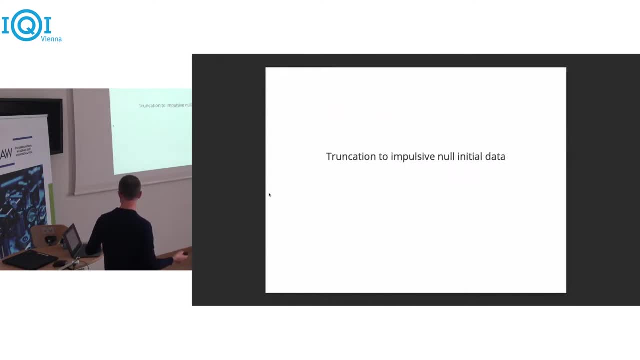 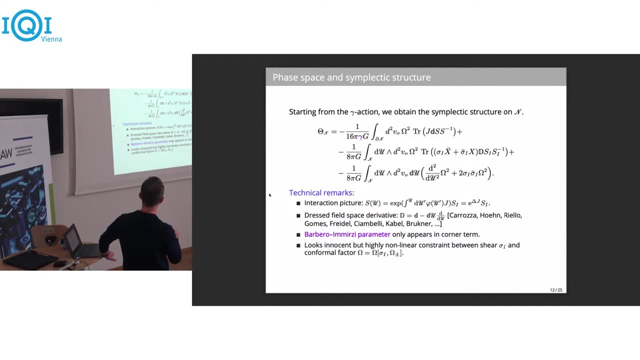 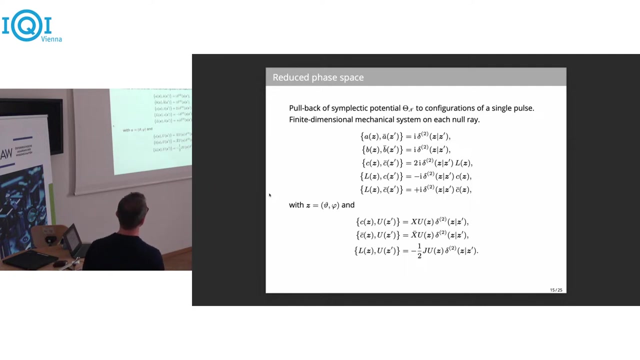 and so both constraints, both equations, simplify for piecewise, constant data, and then you can solve these equations and plug them back into the symplectic structure, and then what you get is an algebra. so in fact, basically two harmonic oscillators and an SL2R. so here the a and a bar. 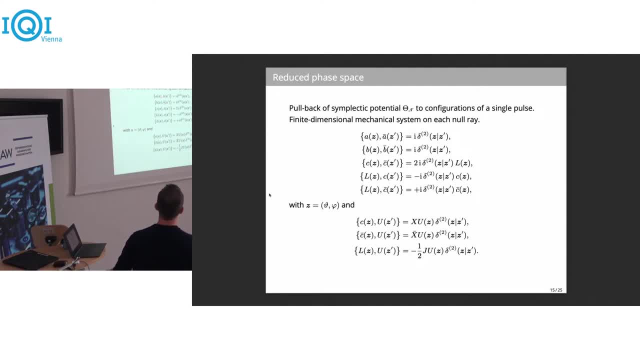 b and b bar satisfy harmonic oscillator, Poisson brackets. and then there is the symplectic structure, for this is the Poisson algebra for the SL2R Lie algebra on the, on the, on the sphere. so theta and phi are our coordinates, and on top of this, 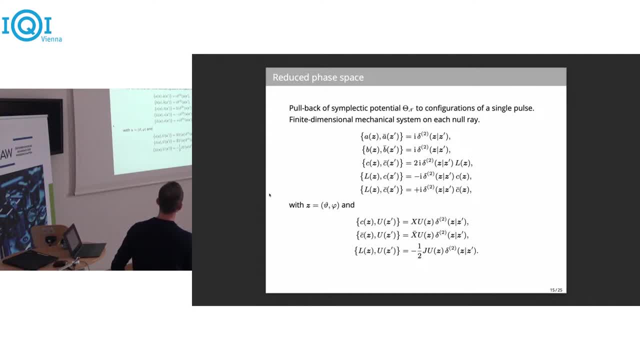 there is a u1, there is an SL2R, Lie algebra group element that satisfies this Poisson commutation relations. so where is all the nonlinearity? now, this seems quite easy. well, it is hidden in the definition of the variables, the relationship between how these oscillators 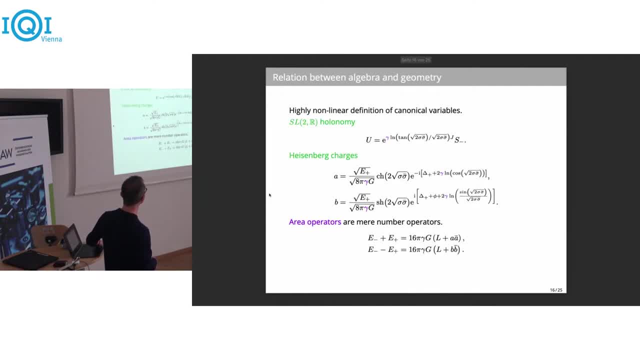 relate to the geometry is a bit menacing perhaps. so the Heisenberg charges a and b, Heisenberg operators. they are related to the area density at the at the future cross-section. the constant shear cosh and sine are hyperbolic cosine and hyperbolic sine. 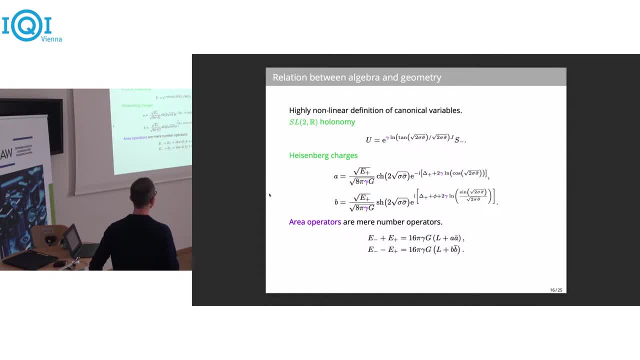 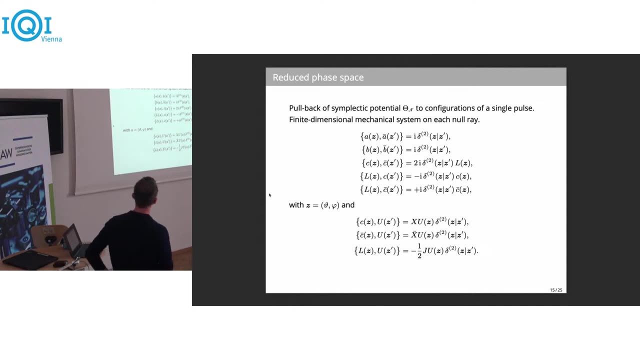 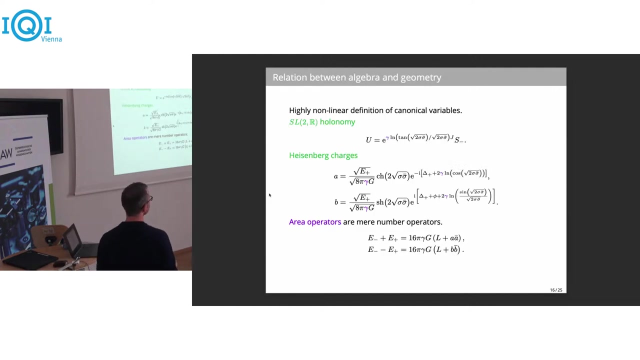 and some complicated phase. however, the area density area at the two cross sections at the initial, the area density at the initial and final cross section, they are just combinations of number operators: l, l in here is the u1 generator, so at the quantum level it will have a discrete spectrum as well, which means that the area density 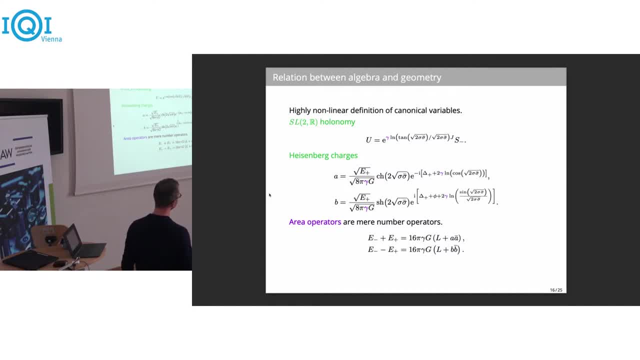 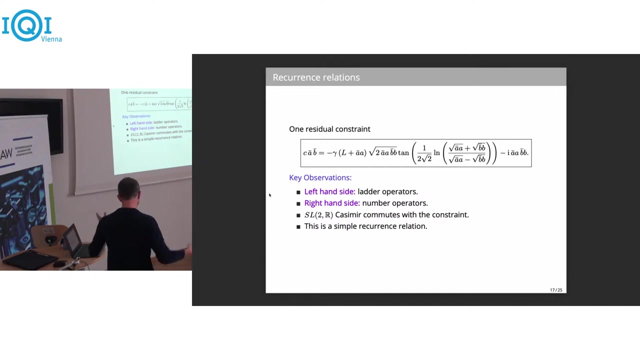 the area of the initial and final cross section, where the pulse either starts or terminates, will have has now a quantum representation and there's an operator that represents it at the quantum level and it is basically a number operator and the shear degrees of freedom they are in this, in these oscillators there's one, if you re-express the constraints in these, 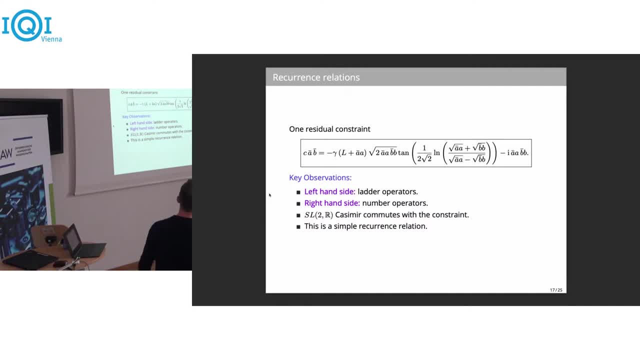 variables, you are left with one residual constraint which is highly nonlinear in terms of these oscillators. however, it has a simple structure. on the right hand side you just have number operators for your oscillators a and a. so a and b just satisfy standard harmonic oscillator. Poisson brackets and c are. c is an sl2r. 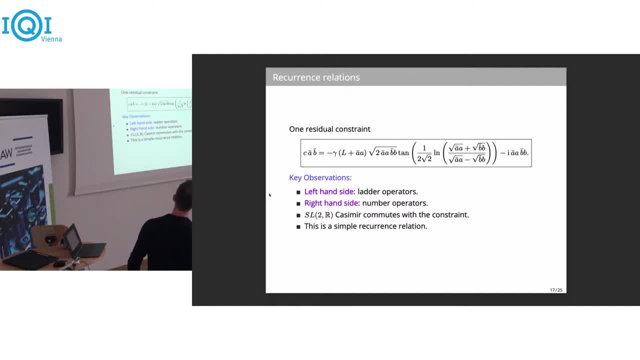 raising and lowering operator. so on the left hand side we have raising and lower ring operators. on the right hand side, we have only number operators. what that means is this is simply a recurrence relations that we can solve and that that is in a way than the end of the 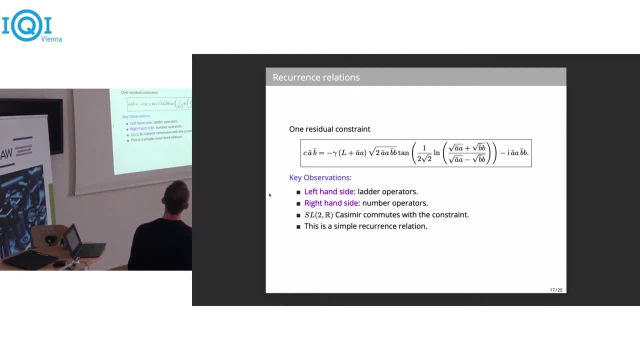 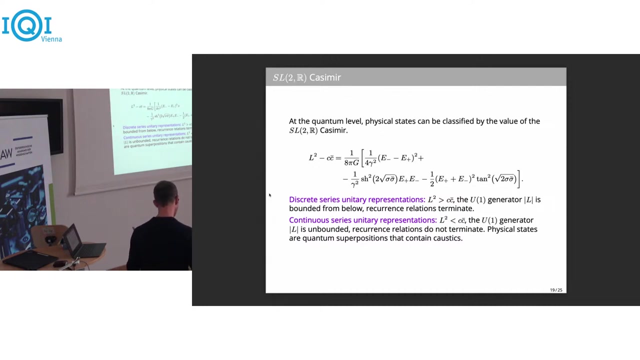 story. so this is: this defines your physical states on the null, on on a strip of the null boundary for piecewise, constant initial data, radiative data. what is also very nice to see is that the constraint generates: so if we have a in here, we have, basically we have to. 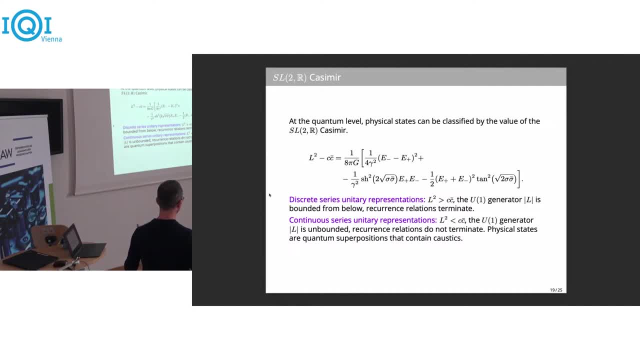 deal with the quantum, with the representation theory at the quantum level of sl2r, where the representation theory of sl2r is characterized by its Casimir. and now we can ask: what is the value of this Casimir and how do we express it? can we express it back into geometric observables, into 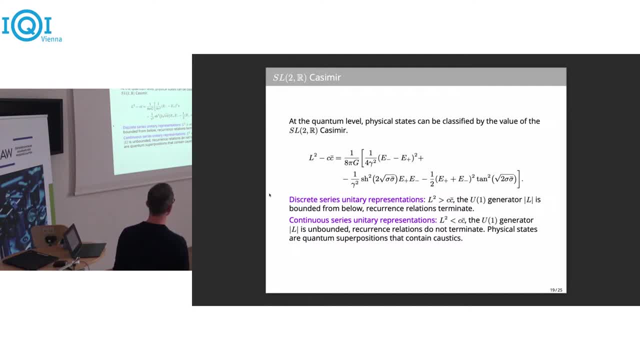 the area densities at the two cross sections and the shear. and the expression that you get is this: and this constraint commutes, this Casimir commutes with your constraints. so it is an observable, so it has a physical meaning at the quantum level. and if the Casimir is, if 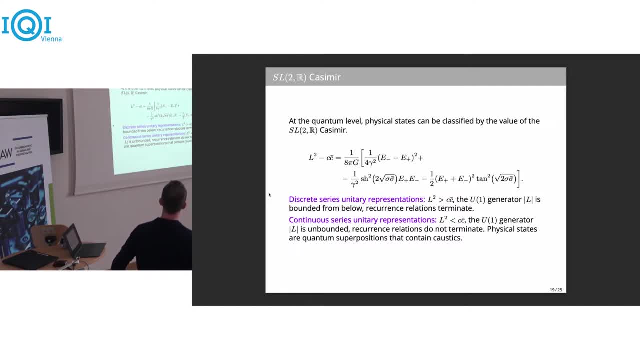 the u1 generator wins, you are in the discrete series representations of sl2r. if the latter operators win, you're in the continuous series representations. so there seems to be a transition happening between two representations: two quantum theories, or two, well two, two regimes, and what? what? 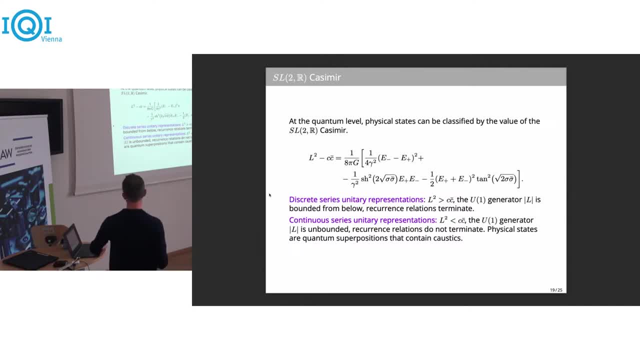 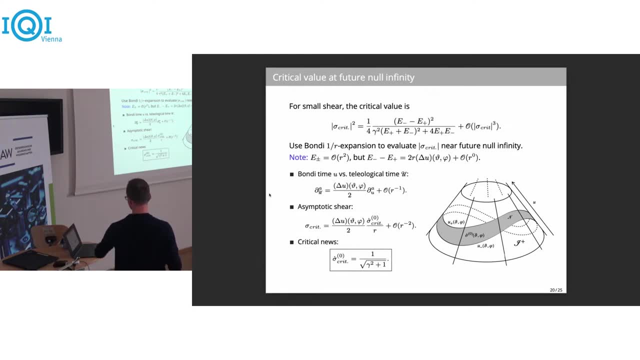 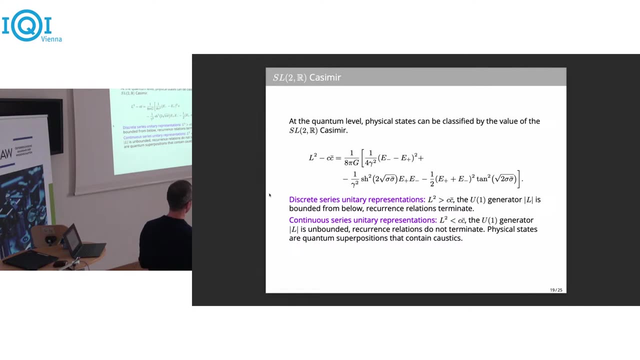 does happen physically, when this transition happens, happen, and what you can now this is this is in this slide. I now take this equation to infinity, so it's. I can now say, instead of looking at such piles at finite distance, what happens if we take. this is a classical, so, of course. now. 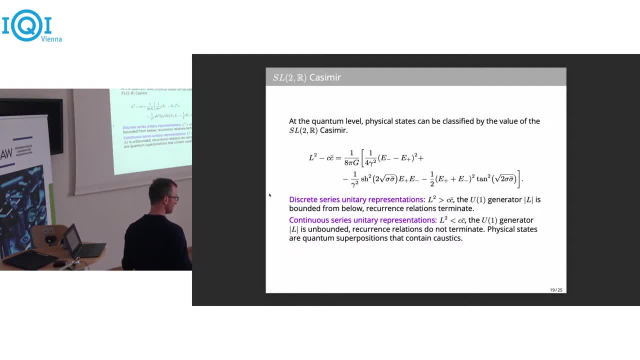 what follows now. the only works on a certain assumption, namely that this has a good semi-classical limit. but if, if the quantization exists and has a good semi-classical limit, then these observers represent just usual geometric data at the now surface boundary, and then we can take the 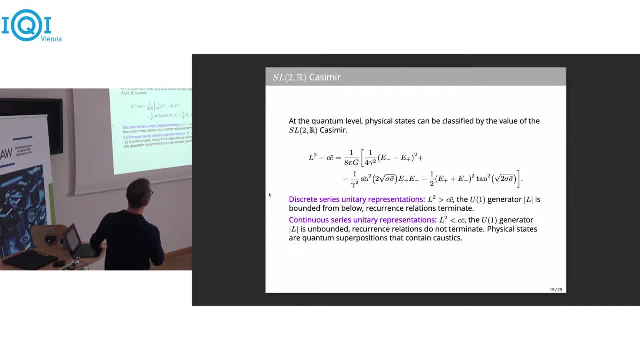 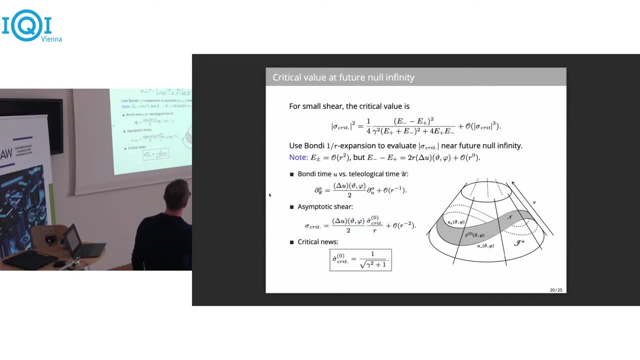 prescription to infinity. take, evaluate or take a pulse of finite duration that intersects future, null, infinity, and what? all? what we then have to do is to relate the variables that we introduced to the standard ones that people use in the asymptotic quantization of general relativity. and then what you feel, what you, what you find, actually is: 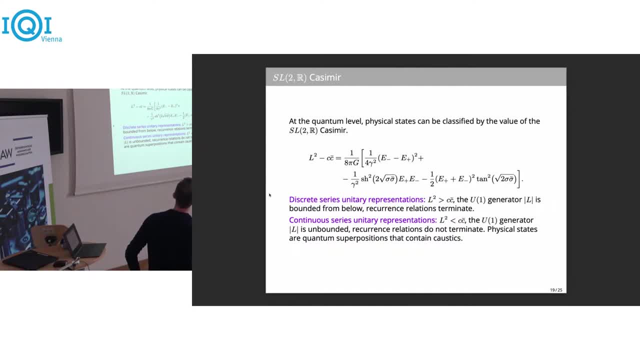 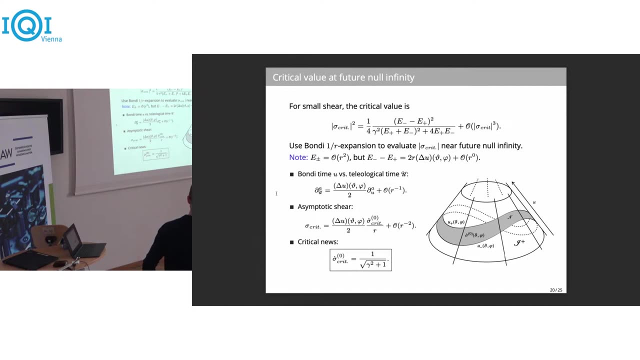 that that the transition happens at a certain critical value of this shear. okay, at which value? well, it's it, it has. the transition between the continuous series representations and discrete series representations happens at the value of the shear. a critical value of the shear, that is just order one where gamma appears. gamma is. 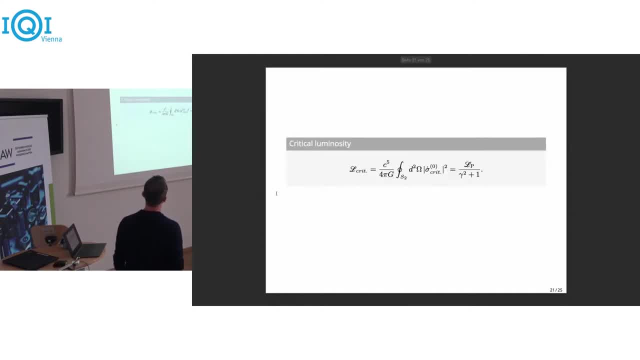 the emersive parameter. and if you now ask, well, these shear degrees of freedom at null infinity, they encode the radiated power. so to what power does this correspond? then it corresponds precisely to the Planck power. so the transition between the continuous series representations and the discrete series representations happens at the critical luminosity, which is of the order of the. 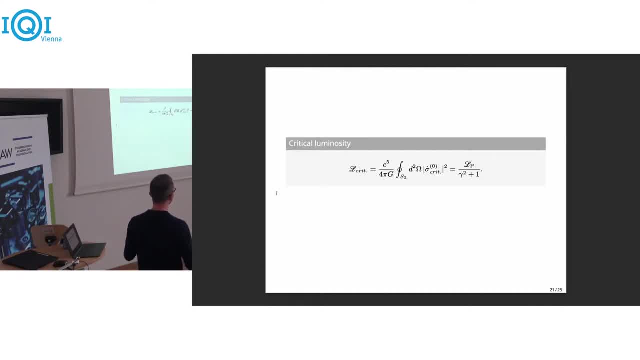 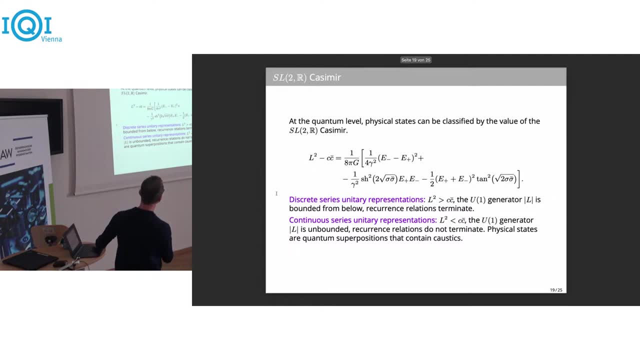 Planck power. this is, of course, only this derivation assumes number of things, most importantly the validity of the semi-classical limit, such that, and if that is true, then we can take this equation to future null infinity and insert the and use just the standard fall of conditions that we know from classical relativity. and if we do that, 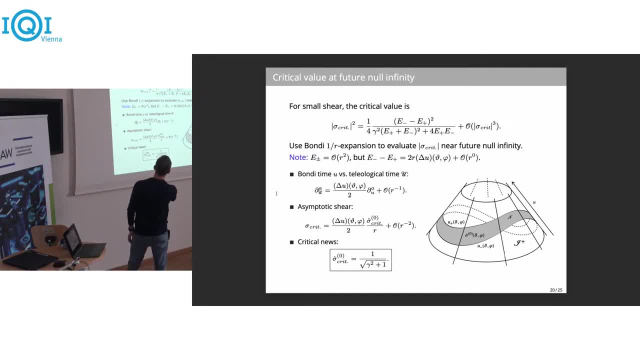 for instance, what one needs to do is to to relate, to find a relationship between the time variable that we introduced intrinsically on the null surface boundary and the asymptotic boundary, the asymptotic bonded time coordinate that we know, that know well from classical relativity and delta U measures, then the duration of the pulse with respect to bonded time. 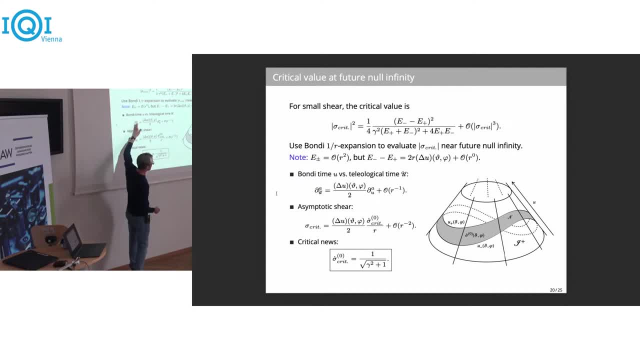 because, with respect to the time variable that we introduced, this has just duration. two, it's just the coordinates, so you can take any value you want, but if you re-express it in this bonded time coordinates, it has a certain. this pulse has a certain duration and this duration also has a certain duration, and this duration is different. 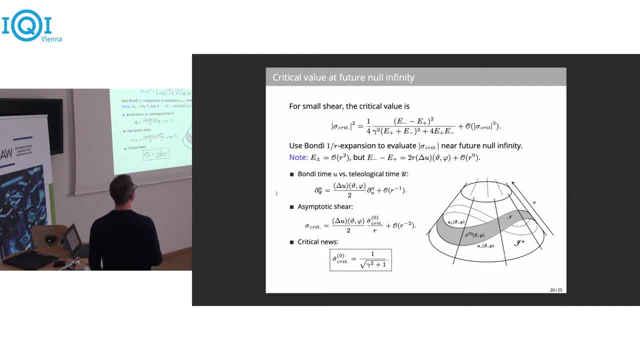 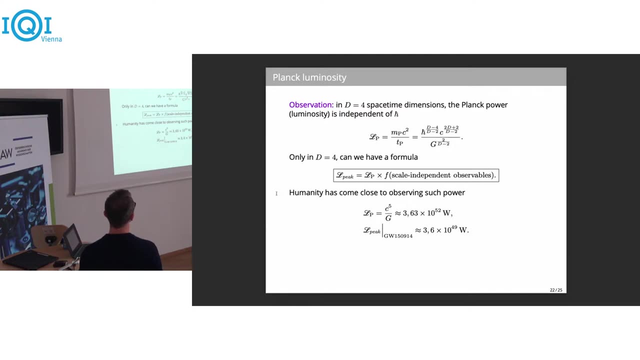 fixes the relationship between the two choices of time to leading order in the one upon our expansion are being the radius, the distance from the source. and what is also interesting is, just as a side remark, that humanity has actually the come close to observing such power, the Planck power. what is the Planck? 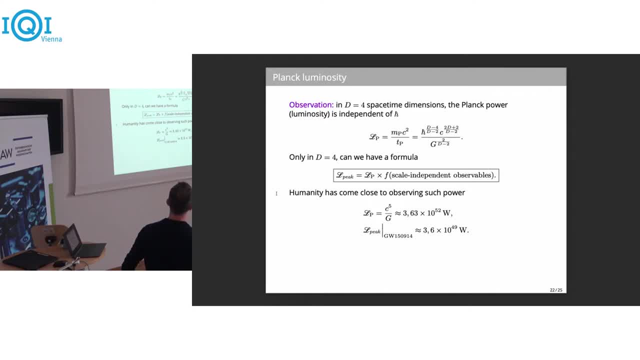 power. the Planck power is Planck mass, c squared times Planck time. if you do the calculation, you can do this in any dimensions. you find something surprising there. in fact, it is only in for space-time dimensions that the Planck power is independent of h bar. in higher dimensions, Planck power does not. 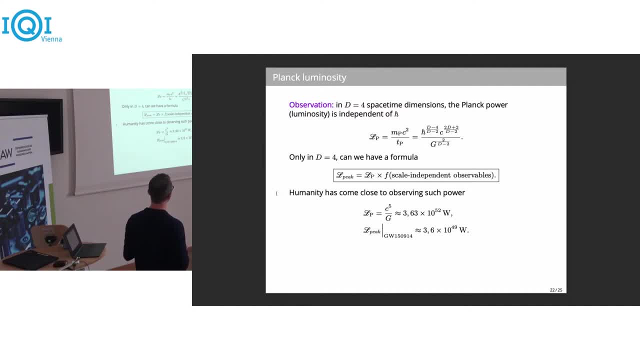 exist. in higher dimensions. Planck power vanishes in the h bar to zero limit. in equal for space-time dimensions, Planck power is independent of h bar and that means that the Planck power can appear in classical general relativity it is, it is allowed to to appear and in fact, if we ask what is the? if we take the 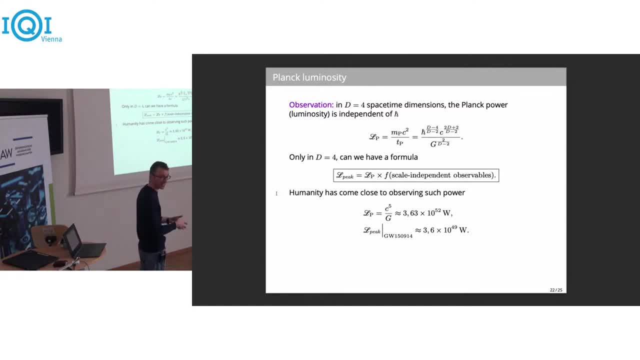 inspiral of two black holes and ask: what is the peak radiated power then? since L Planck, the Planck power appears at the classical level. it can appear also in classical equations, so we can have in d equal 4 spacetime dimensions. 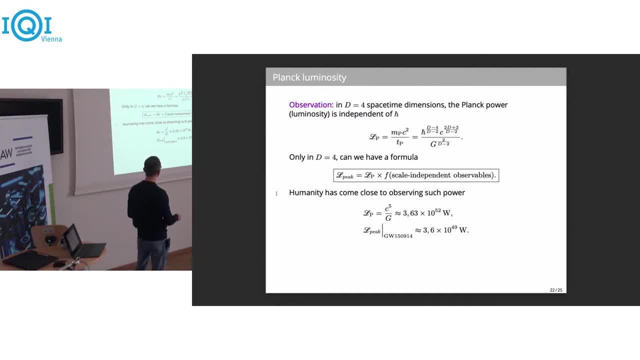 L Planck is allowed to appear. so it is no surprise, therefore, that in 4 spacetime dimensions, the peak luminosity will be of the order of the Planck power. in fact, what we have when we observe the emission of gravitational waves, we are well, we are 3 orders. 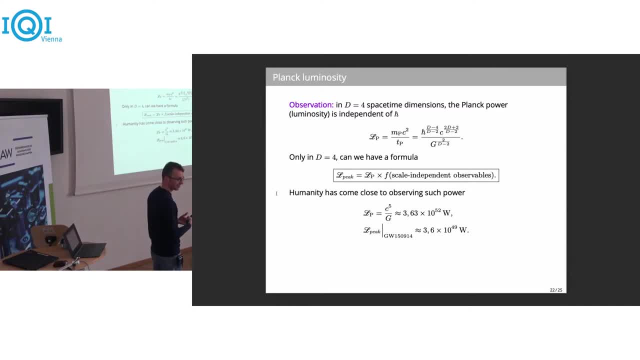 of magnitude below the Planck power. these are the most luminous events that we know of, and what I'm or- the research that I presented to you today in my opinion, suggests that it may be actually possible that there are, that there could be, remnants. 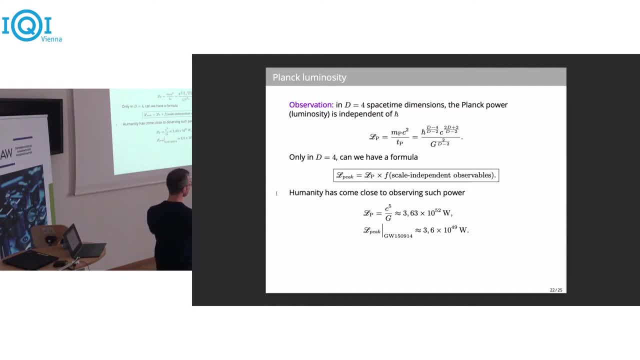 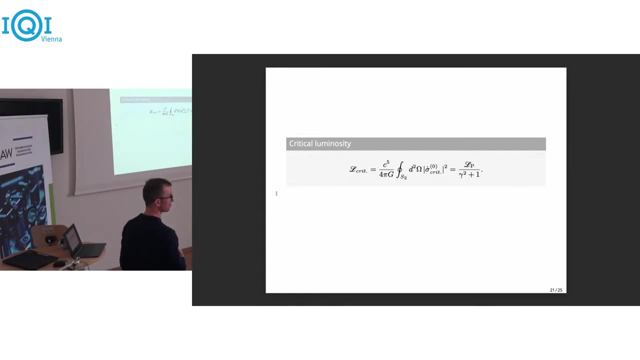 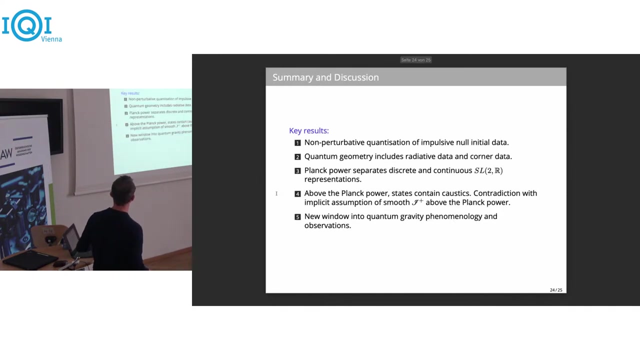 of quantum gravity effects that leak into the classical theory, because the Planck power is close, is the critical power at which something happens in the quantum theory, namely a transition between discrete and continuous series representations. and with this I maybe I give you a a brief summary. 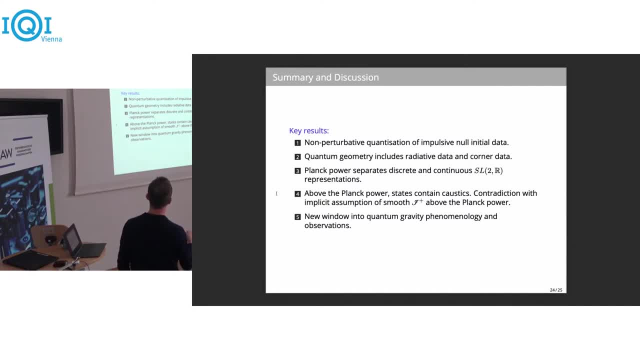 so what we have achieved is a non perturbative quantization of impulsive null initial data, and the quantum geometry that we so found has has a quantum representation of both the initial data. for the Reischauer equation that lives on this four dimension 2 cuts in spacetime. 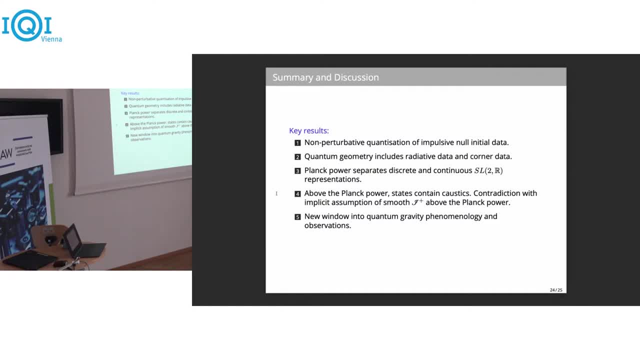 but it has also a quantum representation of the radiative data that can cross the null surface boundary. So this will be quantum, but the data that lives on these cuts will be quantum as well, And the prediction, for instance, is that the area of these cross sections 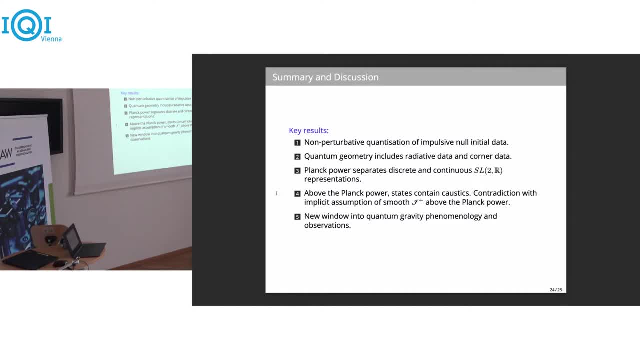 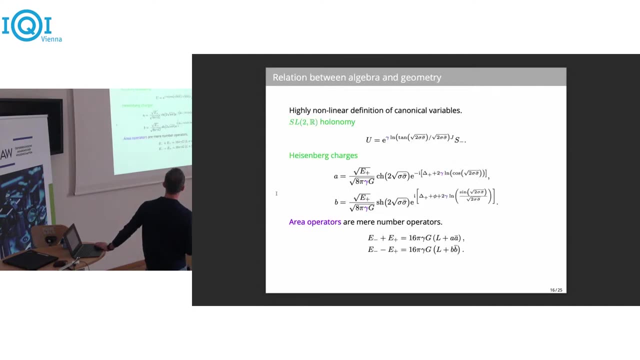 is quantized And this agrees the spectrum, in fact agrees with what we have in lukewarm gravity, that the area. so here I said that the area densities at the two cross sections is basically a number operator where the immersive parameter now shows up. 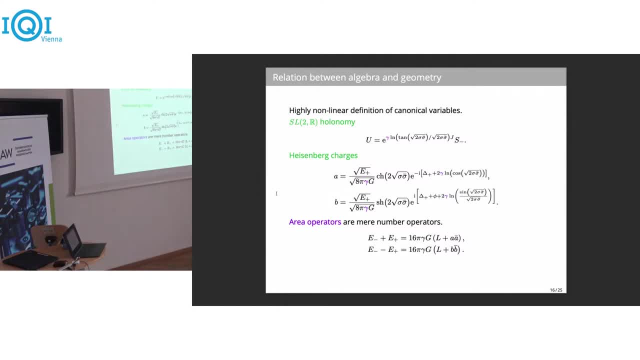 And this is just what I said earlier- that by introducing the immersive parameter, what we add is the. what is deformed at the quantum level is what's happening at these cuts. So this has physical effects. Okay, if we turn on gamma. 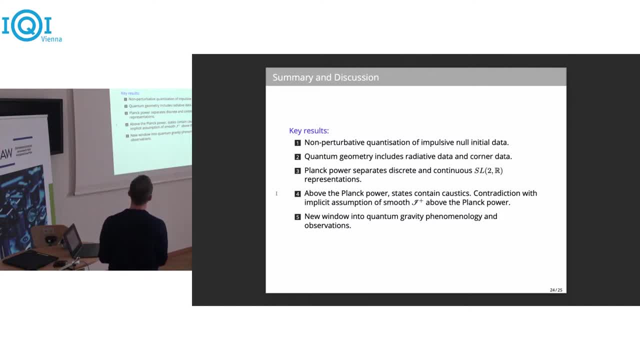 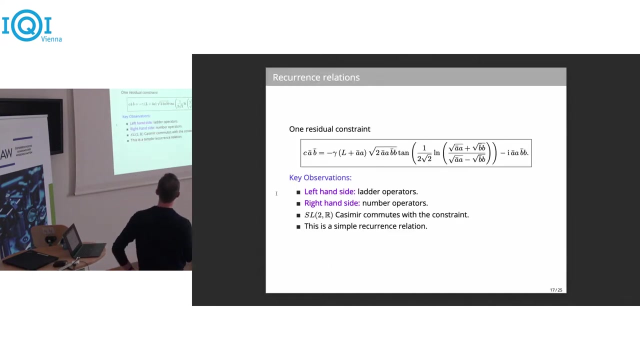 And then something seems to happen. I have only indications for that that come from. Well, actually it's a bit stronger than that, But what I find is that if we are in the continuous series representations, then what happens is that something else happens, I should tell you. 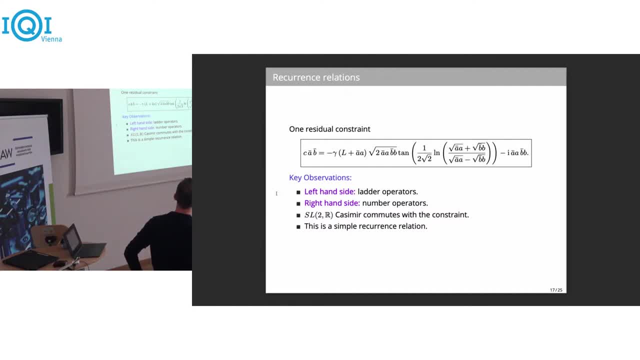 So for the discrete series representations, these recurrence relations can be solved very easily. It turns out that you only need finitely many. These terminate at some point. And they terminate because of the representation theory of SL2R. So C and C bar, they are like L plus minus for SU2,. 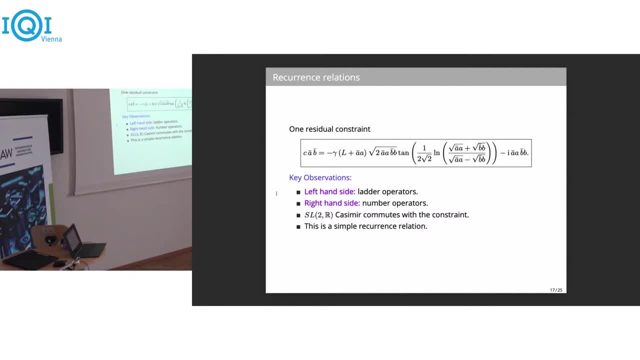 just that. in SL2R it goes in the other way. There is a minimum magnetic quantum number and the creation operators go up, And this minimum for the magnetic quantum number means that this or implies that these recurrence relations terminate with finitely many states. 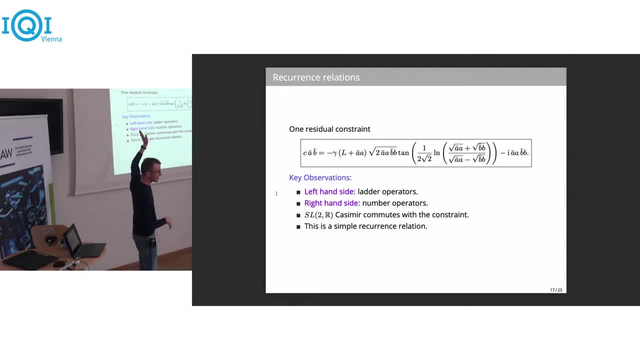 But for the continuous series representations, this doesn't happen, and you have to sum up infinitely many states, infinitely many states in which the quantum numbers for A and B become infinitely large, at which point the shear degrees of freedom diverge. 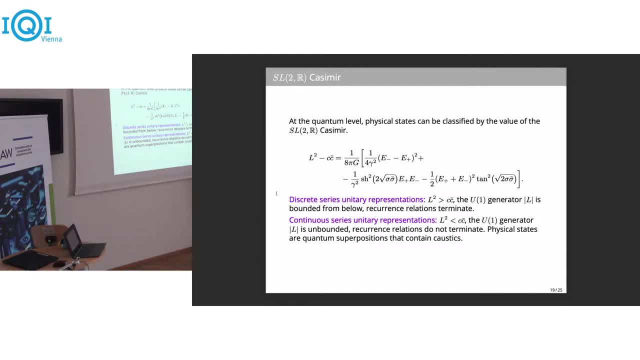 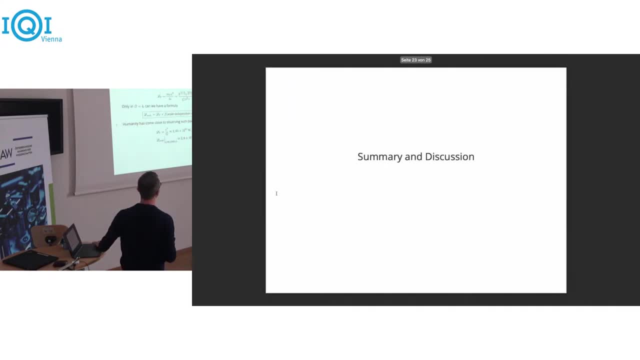 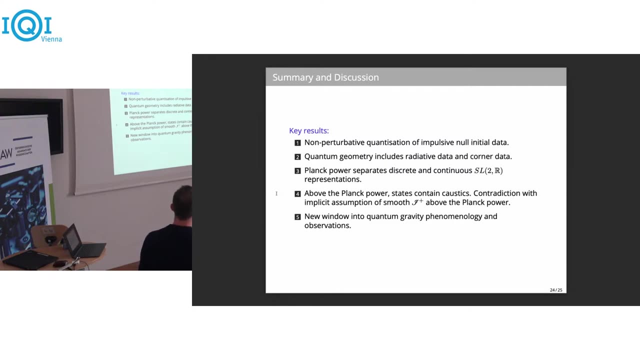 which then implies that you can create caustics, And this can be avoided when you are working with discrete series representations. But for the continuous series representations there seems to be a problem, which suggests in fact that the, the theory at 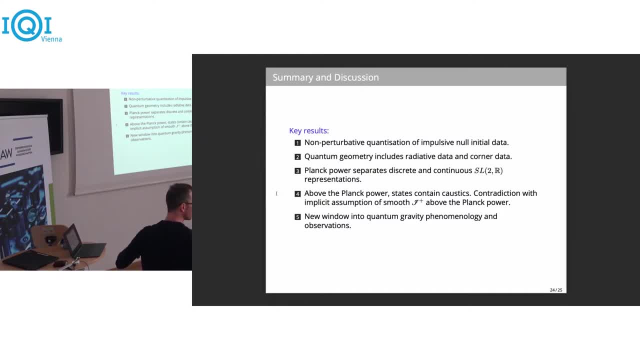 at square at future, null infinity will be governed by the discrete series representations, And what I hope is, and what I want to explore, is that this can provide a new window into the quantum gravity phenomenology That the emission, for instance, the emission spectrum. 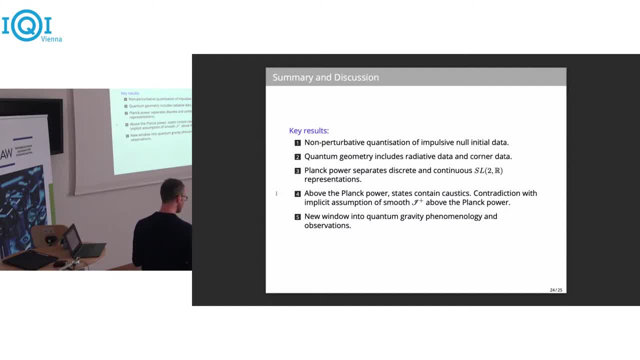 of a gravitational wave, that there will be some fine structure of the emission spectrum of gravitational waves that will be governed by the, by this immersive parameter that can show up then in in physical, have physical implications. Thank you, Thank you, Poulpen. 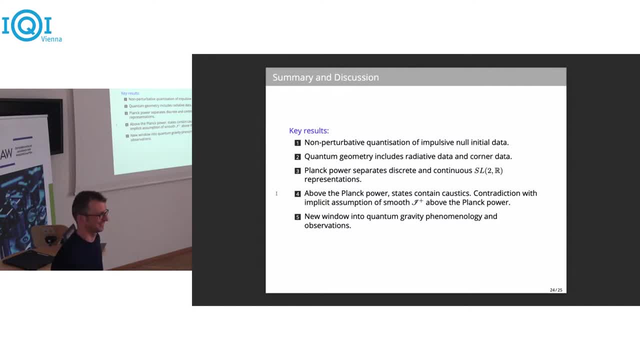 Questions. Thanks for the next talk. The emitter curve or anything else aside from what we presented, like the K-ISR speculations, it could be large so that the be closer to what is already observed, or something like that. 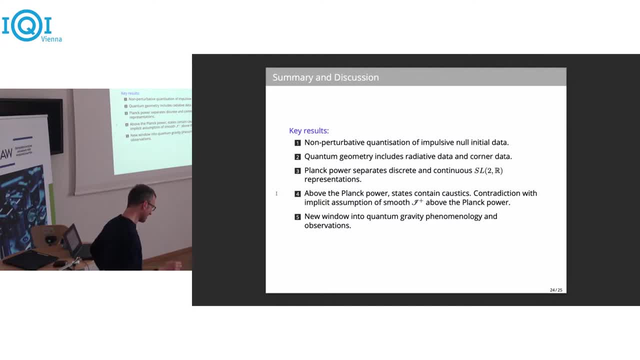 Mm-hmm. In fact, the immersive parameter sets the fundamental scale in loop quantum gravity, Just like here. we have a transition happening for the luminosity. in quantum cosmology, for instance, what one finds is that there is a maximum energy density given. 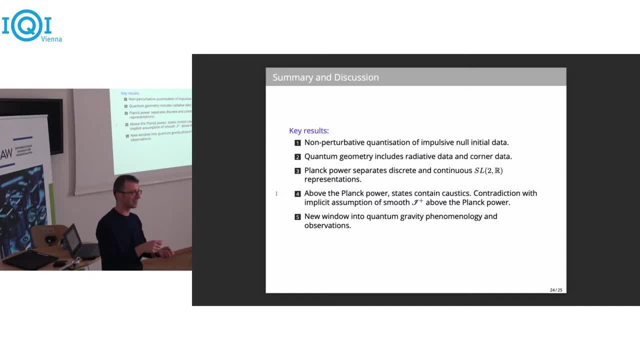 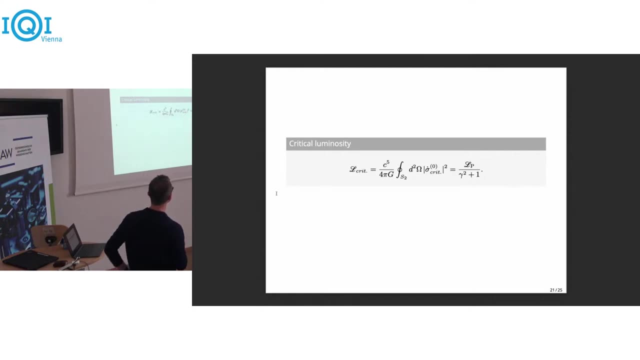 by the Planck energy density And the relative, which then depends on the immersive parameter. But of course there is a more trivial, more immediate result. In fact, if gamma would be, gamma cannot be arbitrarily large If gamma goes to infinity. 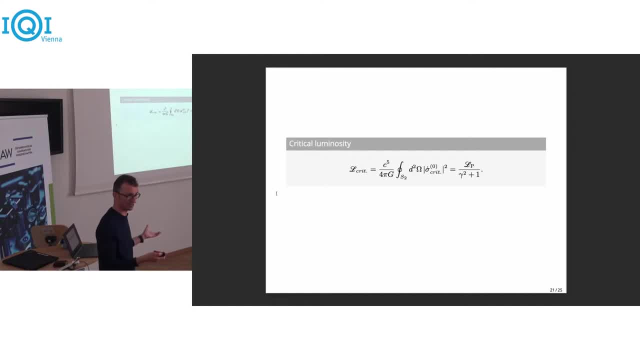 this transition goes to zero, But we have observed gravitational waves, so there is already a constraint on gamma from there. Yeah, Great, Just a very Yes Is the continuous representation above or below the Planck power. Above, Below Planck power you should have. 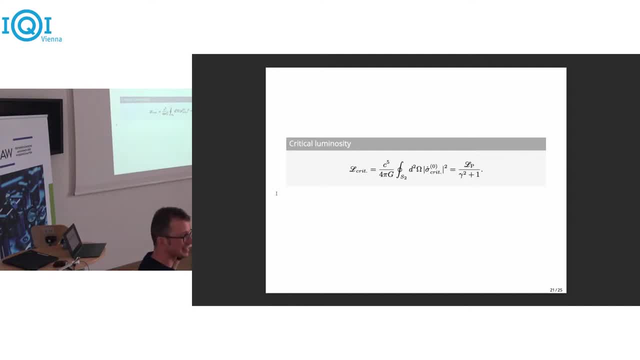 the discrete, Yes, But there can be many, many states, You know, because it's not that just because of discrete series representations there are not. The immediate concern could be that there are not enough states That this would be in conflict with. 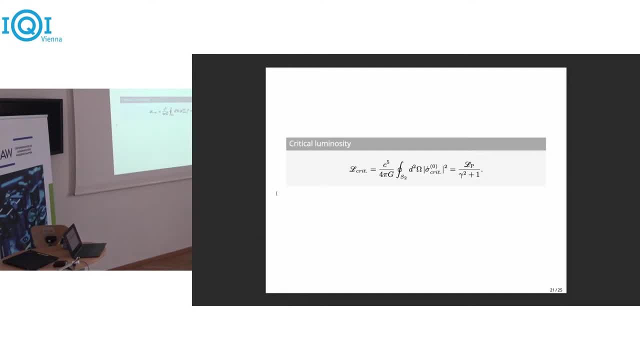 That the Hilbert space is not large enough, But remember that there is also now a Hilbert space for this. data at the corner, at the cuts, the two cuts. And what is How? What determines the size of this Hilbert space? 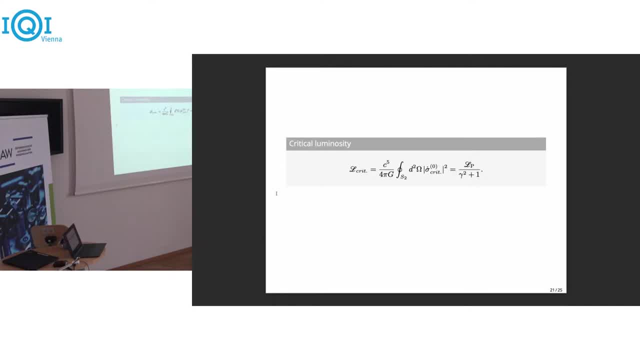 Well, this Hilbert space is characterized by the, Or characterizes the area of the cross-section. So if the area is very, very large, then many, many states, So the, But it's true, below the Planck. So what? this analysis? 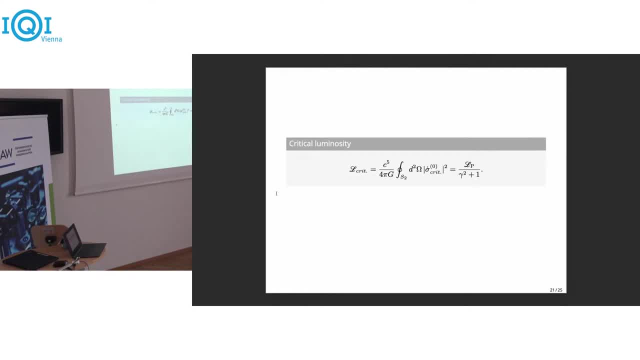 shows is that below the Planck power, the spectrum of the emitted power would be. The spectrum of the power that such a pulse carries would be Would be discrete. You mentioned the representation for SL2.. Is it only bounded below? Is it bounded below as well? 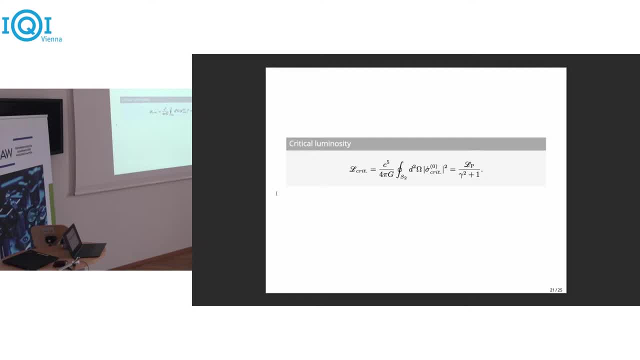 No, Well, if you quantize SL2R, this is unbounded, But not all states are allowed, because there is a constraint, A constraint that links the quantum numbers for the area to the quantum numbers for this SL2R. So 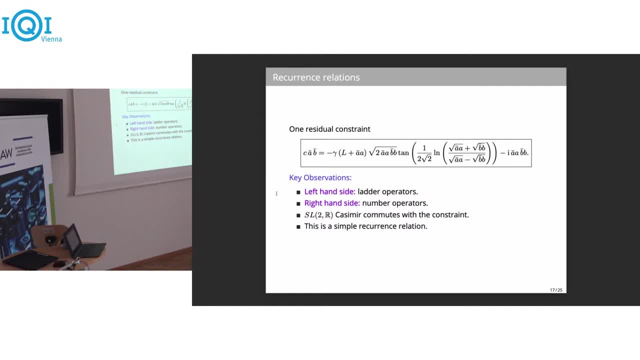 And what you get is a recurrence relation that goes down. And so you start from some maximum state with some magnetic quantum number- n, c, let's say- And then quantum numbers for the two oscillators, And then you go down, And then it stops. 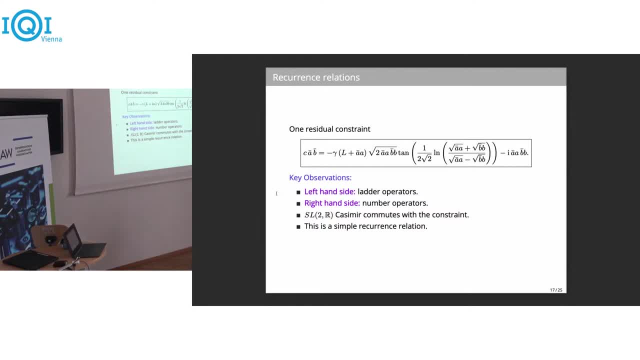 I see I understand what you're talking about. Any other questions? Can I ask something more kind of criminological? So you said that this will use the surfaces of, of the, of the or some rupressions. 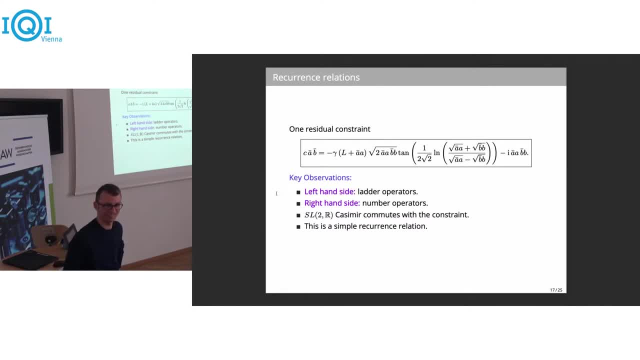 Am I right? Yeah, This is just quantization of light cones. It has nothing to do with the light cone itself. Up here I mean: Okay, I can imagine many different light cones, but every surface on this light cone should be. 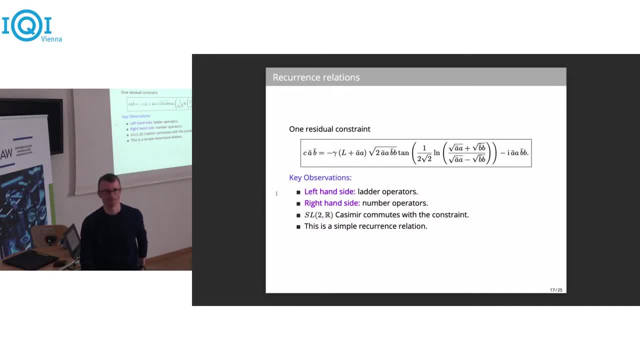 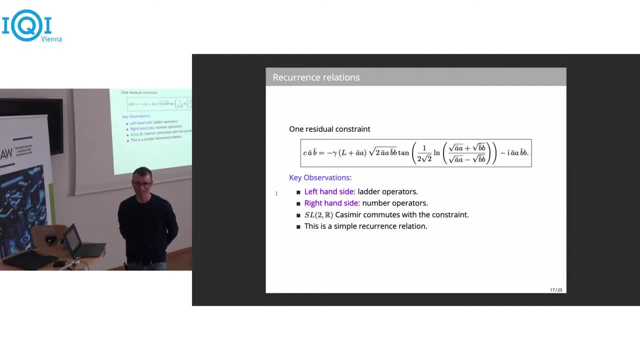 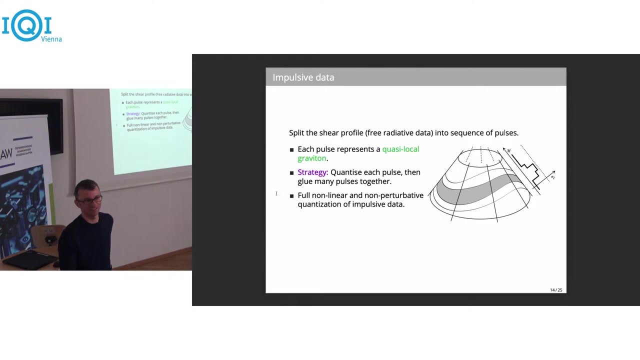 your question hints at something I think. no, no, no, I want to continue. it hints at, sorry. it hints at an implicit assumption that this program relies on, namely that it makes sense of that, that it is sensible to speak about such surfaces at the quantum level, which which? 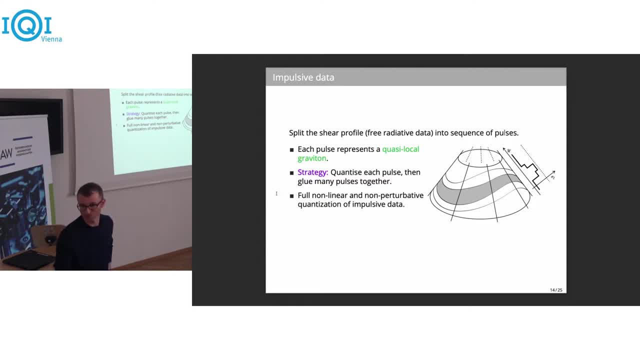 relies also on the assumption that the speed of light is that there are no fluctuations of the speed of light, in that sense that there is no, that these surfaces can be sharp. and now you may ask: is this perhaps in conflict? well, I, I would say that one. 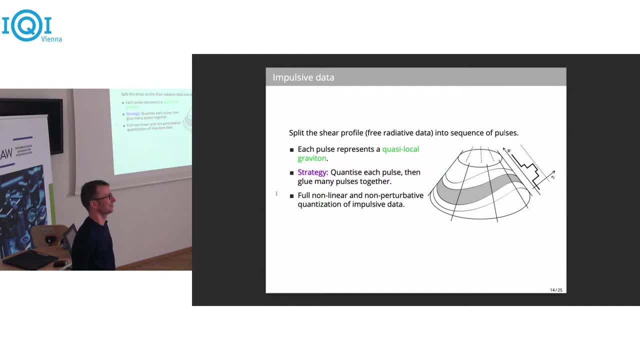 one one. I would say that you, you could imagine coupling matter in here to this, to gravity, and define then light propagation, and, like we would do it in an experiment, operationally. so we measure, we want to check whether, for instance, we want to check whether the speed of light 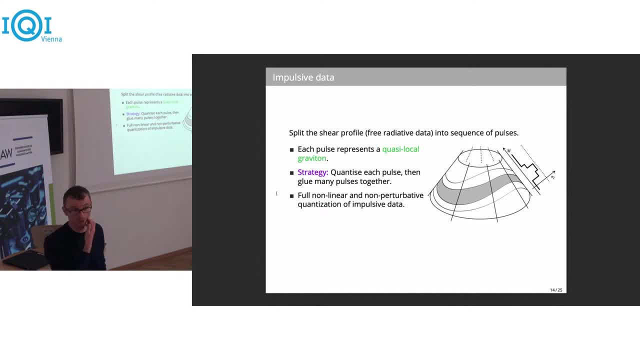 does not depend on the frequency. so we would have to add, we would have to set up an experiment and then ask: how does this experiment translate into this formalism and do we get some deviations? this could very well be, I don't know, because this is a very difficult question. 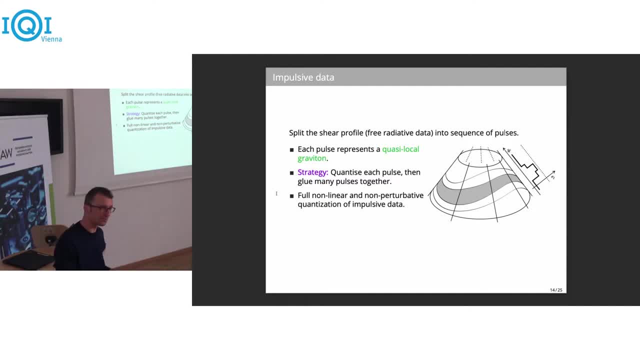 so this is not a priori assuming. assuming a light cone structure at the quantum level like that is not necessarily in conflict with observing deviations from the speed of light in physical experiments when you do, when you use physical rods and clocks, because physical rods and clocks may. 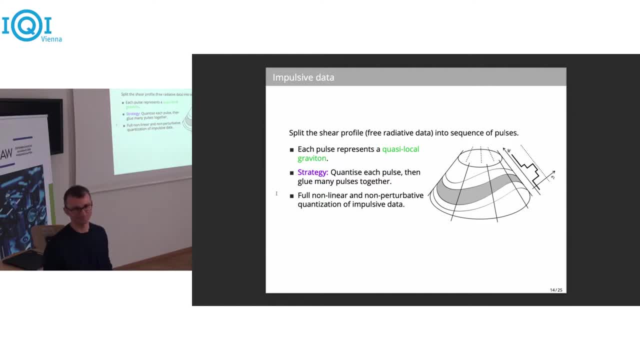 add additional effects. but yeah, I think, yeah, I just want to check if my understanding of this discussion is correct, so I don't know much about this, but is this kind of whether this way of surface quantization is a more intelligent version of this municipal space? so, municipal space. 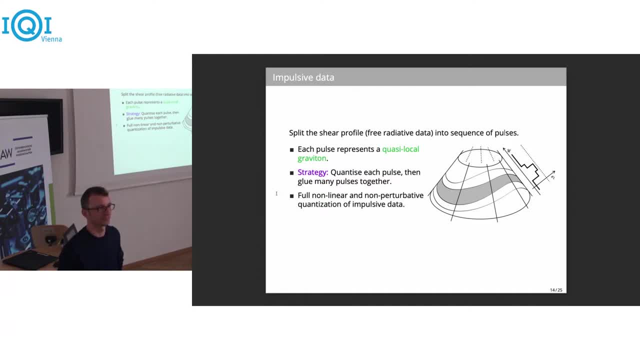 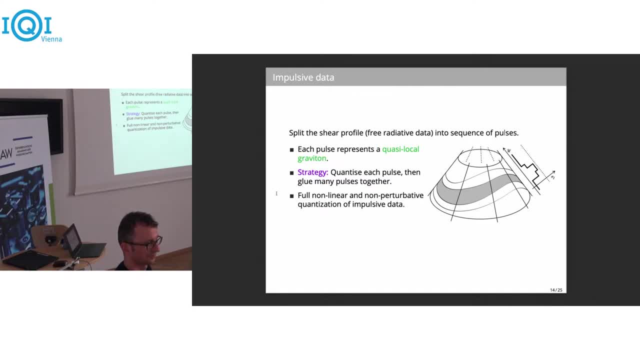 with quantization, just with handling your systems and the new model, and I always ask myself if such a discussion existing in quantum, if you can reduce dimensions or reduce your space, if this is, if this is compatible with to ask quantizing, and then yeah, so yes, this. 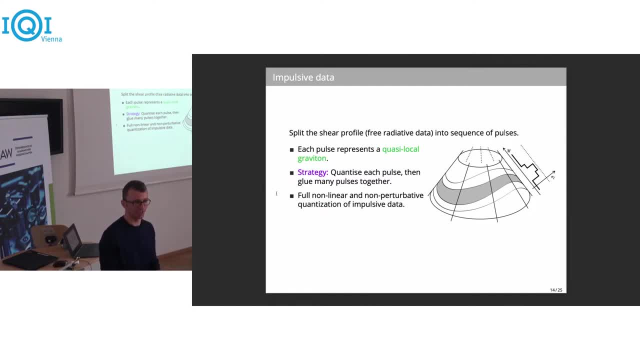 the starting point is a truncation. a truncation where along each light ray, you only have finitely many degrees of freedom. still, there are infinitely many degrees of freedom, of freedom in the angular directions. in fact, I should have also mentioned that the face basis is, in a way, ultra-local. 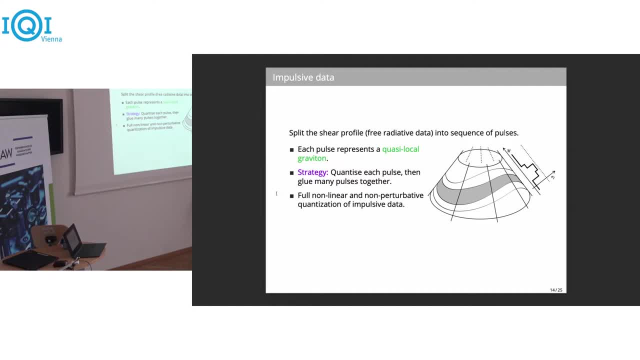 in the angular directions. so different points at different points at different light rays are all space-like, separated and mutually commute. so the algebra in the angular directions is ultra-local. but this this goes away a bit away from your question. the question was about the like symmetry reduction. 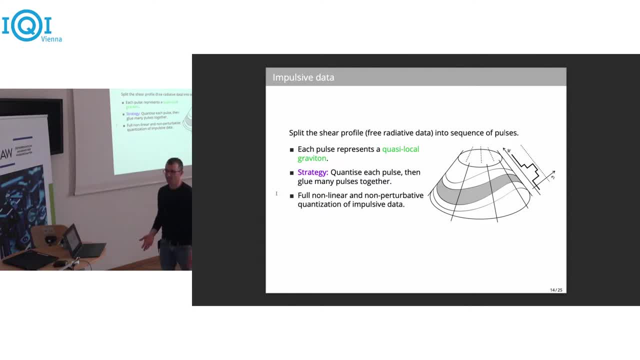 and mini super space. so, yes, I would say, all physics at some point relies on a truncation. so we do whenever we, for instance when we do quantum chromodynamics, we use a lattice to perhaps even define the theory. so all physics relies on some truncation. the question is then: 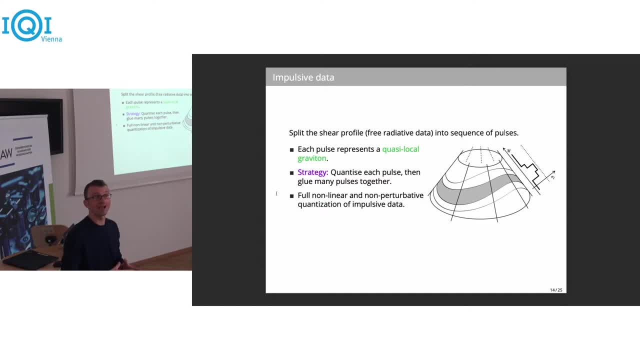 how to, how to go back to, how to go back to the continuum or how to go back to to arbitrary initial data. if you do a mini super space quantization, it is not that you can glue many universes and get a approximate to arbitrarily good precision, any. 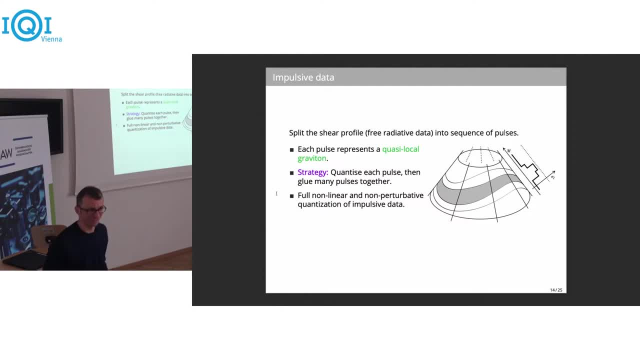 uh any other solution. this is kind of obvious. but here here we are in a different situation. when we are using step functions we can use to approximate to arbitrary good precision any smooth uh function with respect to uh to the usual standard L2 inner product for the. 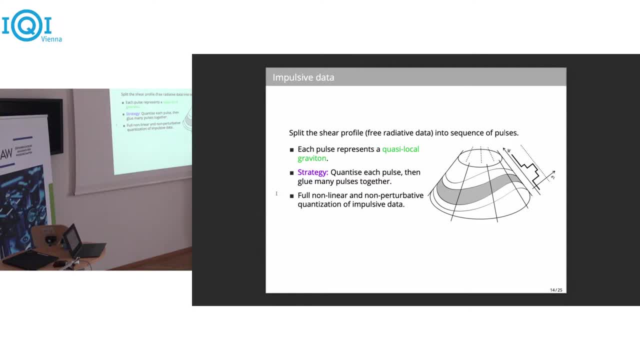 for the initial data. so we are in a. so this is a different kind of truncation, i would say, one that is uh, uh. of course you lose smoothness, but otherwise you can, in the limit where you have infinitely many such pulses, and you stack them. 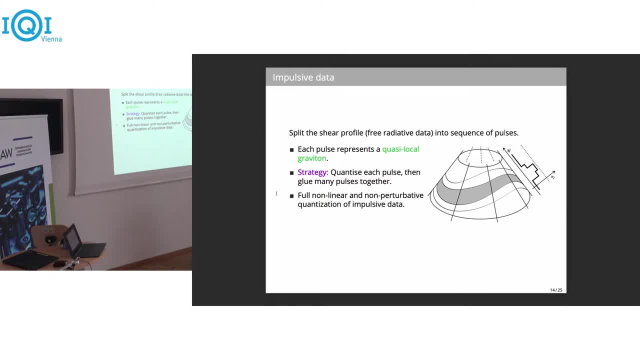 stack them together. you can still reach any point in the in phase space, in phase space for the radiative data. okay, i think we can conclude at that point. thanks, thank you, thank you.